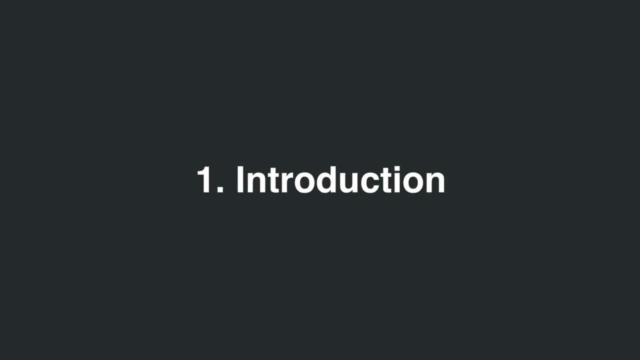 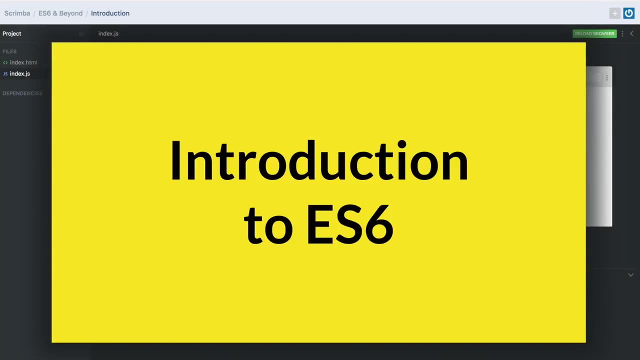 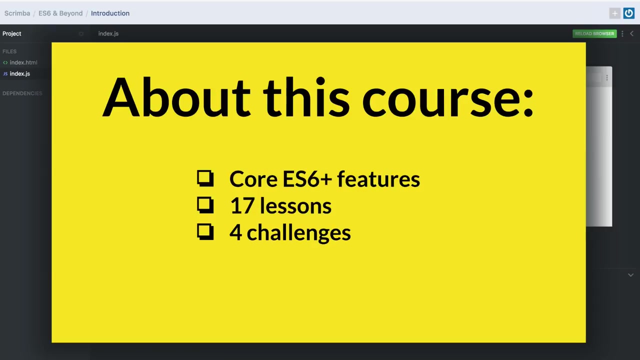 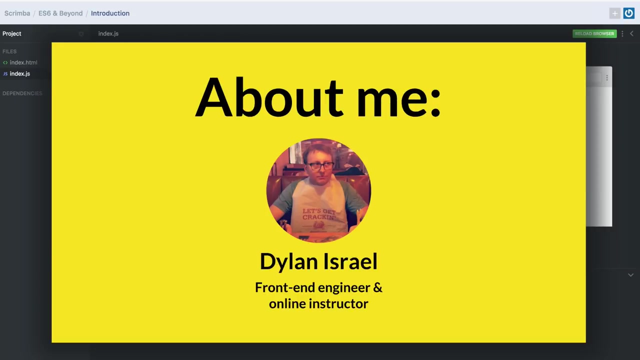 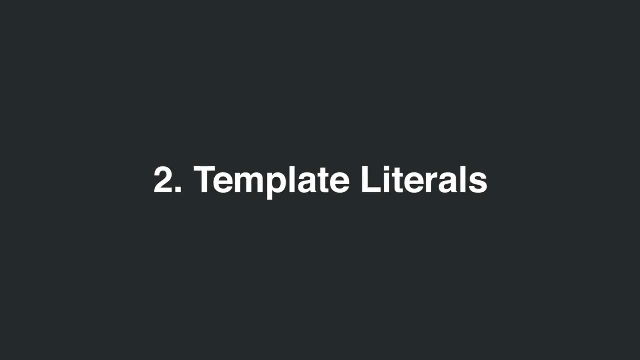 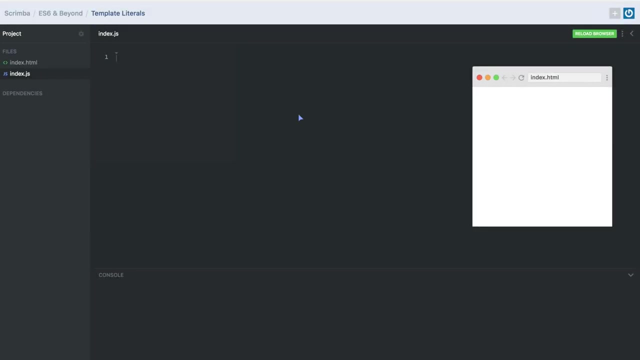 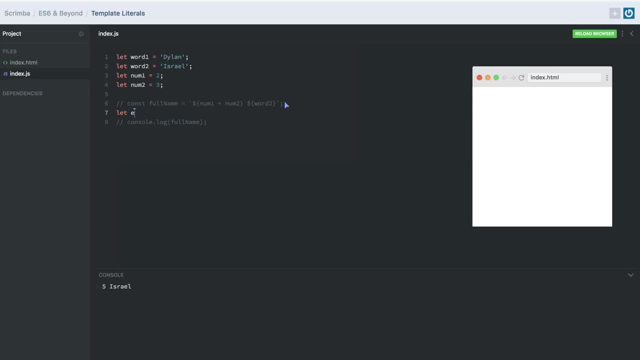 Let's go ahead and comment this part out here and we'll create this variable called example In the past how we would have to do a multi-line string. we'll do hello, world, Hello, and then we want world to be on next. 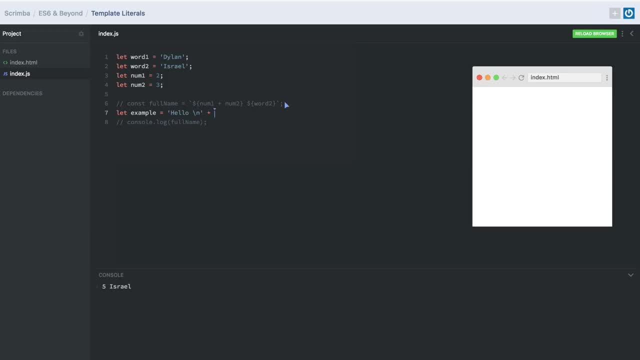 We'd have to escape with a slash, and then we can go ahead and add world, Like so, And then, because of the way that console log works, it's not going to actually showcase it here. As you'll see, it's going to print it out on one line. 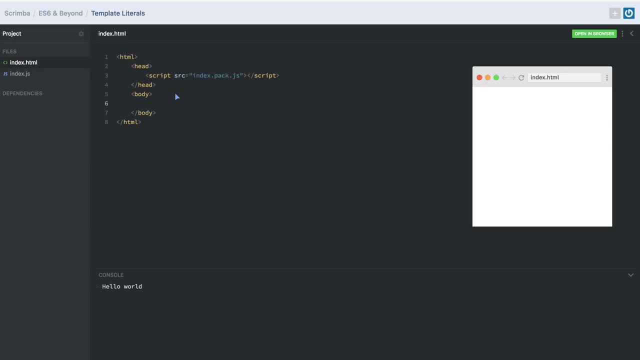 So what we'll have to do is we'll jump into our index HTML and create a little paragraph tag, And what we're going to do is we're just going to give it an ID equal to example And then in our indexjs, instead of console logging, we're going to go ahead and just target that. 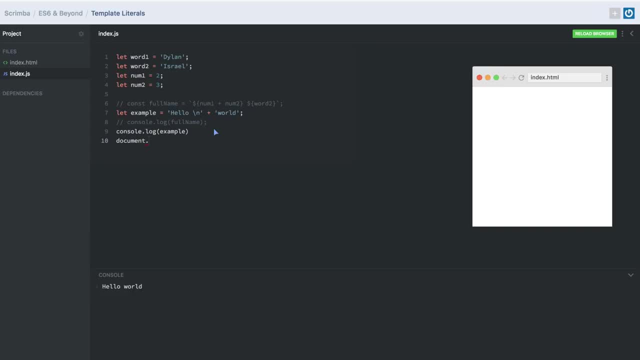 so that we can actually see it Being on multiple lines on the page. So we're going to say document: get element by ID, And then we're going to say example, which is the ID on the page, And we're going to set this equal to our example variable. 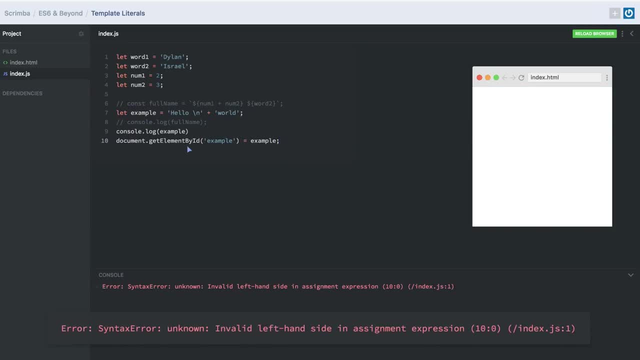 So go ahead and save it. Excuse me, dot inner text, because we're trying to set the text value of that- And then you'll see hello world on two lines, Although this slash n is really sort of obnoxious. So how can we go about fixing that? 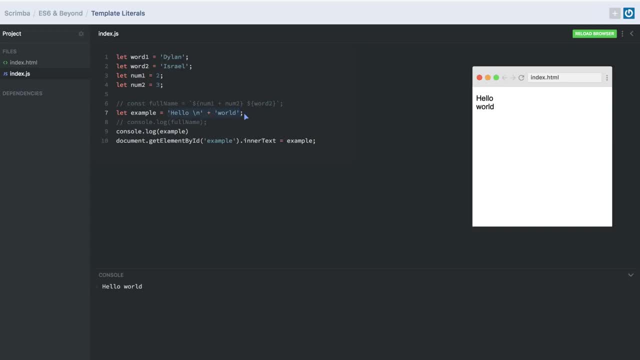 Well, let's go And use our variables here with some string, with our some template literal. So we use the back text And notice, on the first line, here I'm going to put my name, which would be word one, And then on the second line, I'm just going to go ahead and put word two on here. 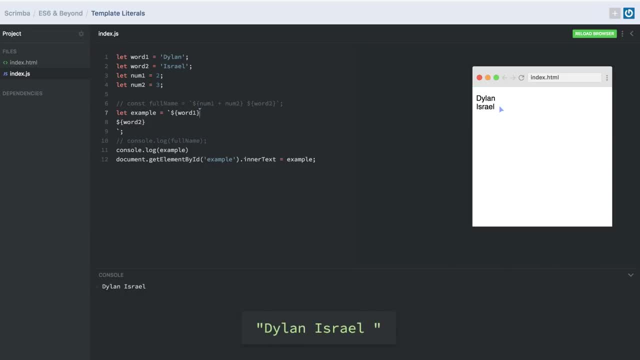 And us formatting our string like this will also get Dylan Israel on multiple lines, And if we obviously didn't want that, we could do it on one line as well. But it allows us a very easy way, a very clean way, to have multiline strings. 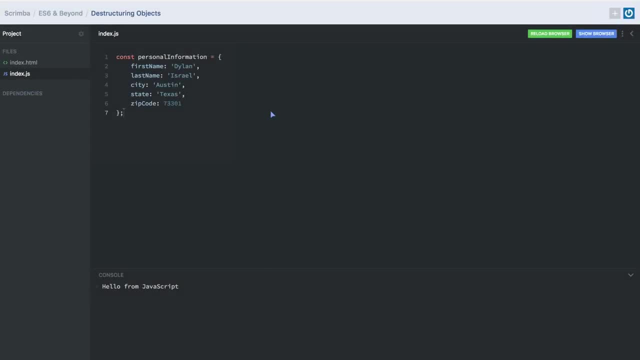 One of my favorite additions to the JavaScript programming language has been destructuring objects. So see, here we have this personal information object with first name, last name, city, state, zip code, a bunch of stuff. Now, what we want to do is, or what destructuring objects gives us. 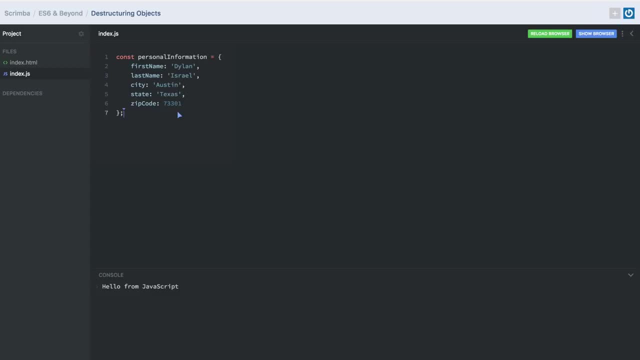 The ability to is. it gives us the ability to essentially write shorthand code as well as reassign values. What do I mean by that? Let's go ahead and create a const here where you'll see we have this opening and closing curly brace And what we want to do is we just want to put first name. 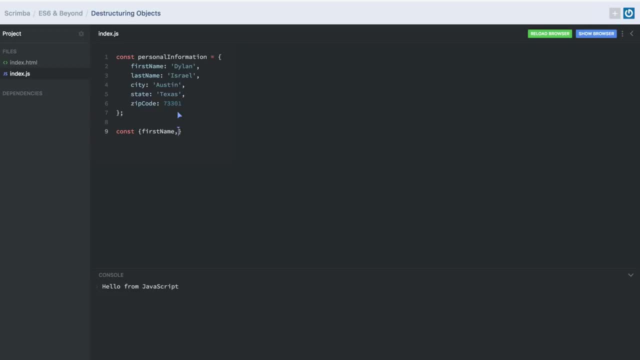 We want to access first name because personal information dot first name Every time we want to use it. that's kind of a pain. It's kind of a long name. We want to access last name and anything And we could access every property on here if we want. 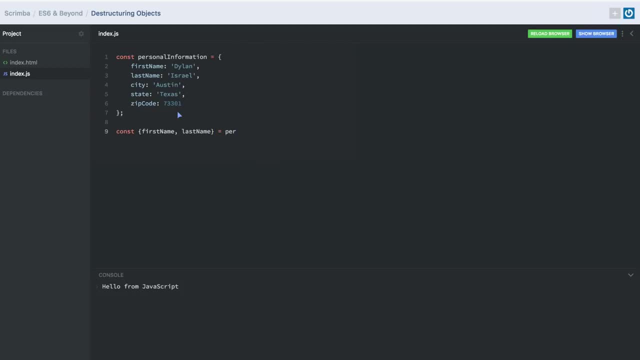 And on this Side, we're going to go ahead and just set it equal to the personal information constant. Now say, what that's going to give us the ability to do here is: And let's go ahead and use some template literals or string string interpolation here. 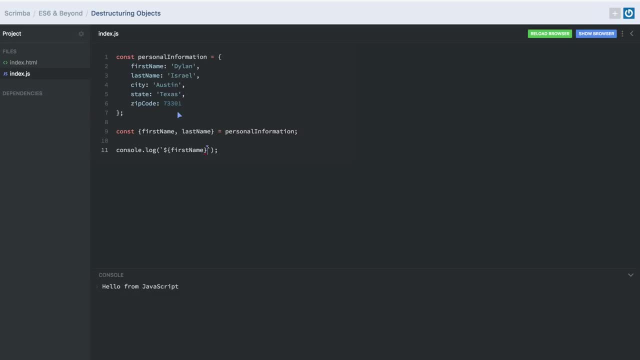 And it's going to give us the ability to just do something like this: We're going to do first name and then last name And it's going to print it out like so And we don't have to do personal information- First name- every single time we want to use it. 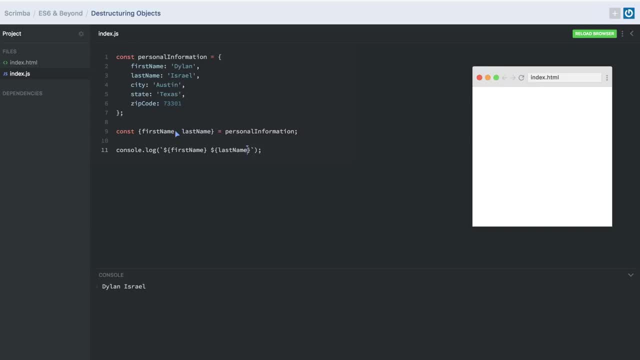 But we can actually do one step farther. One step further than that is say we wanted to actually reassign the value here. We just put colon and put FN for first name and colon LN for last name, And we could replace this and put FN and LN to hit those values as well. 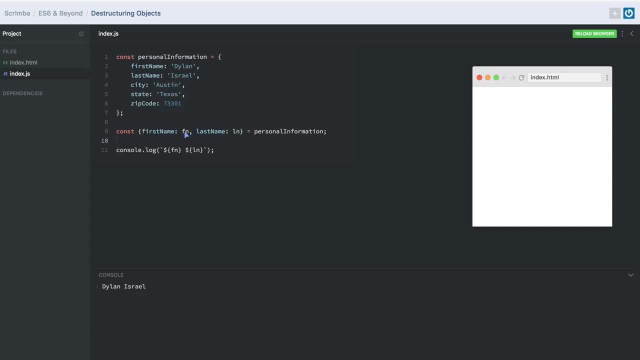 You'll see we have first name and last name. Now I would say that if you are going to rename something You know, make sure that, when it comes to naming convention, it makes sense. Or if you're going to do very short names, like this in this instance, make sure that you follow good naming. 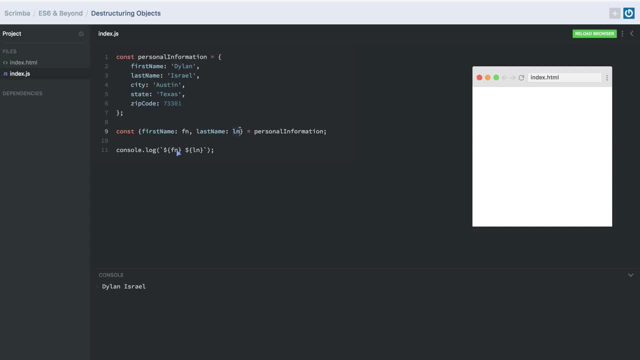 Not only good naming convention, but also make sure that the scope of it is very short. But this allows us in general to destructure our objects so that we can have access to these things, And we'll talk a little bit about how we can destructure arrays in the next video. 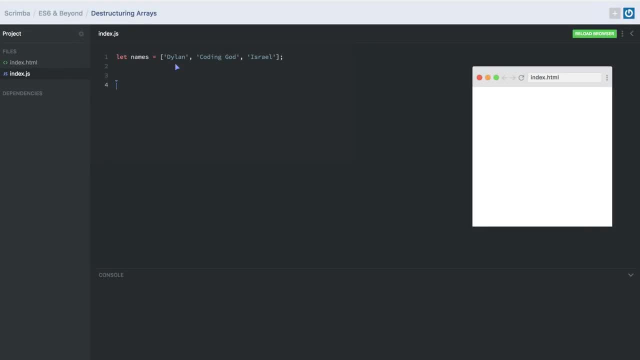 Destructuring arrays is another great feature that's been added to JavaScript in recent years. It's very similar to how we destructured the objects earlier. So we have this name array And what we want is to essentially create a pointer element to destructure our array so that we can get the first name, the middle name, the last name, in this instance. 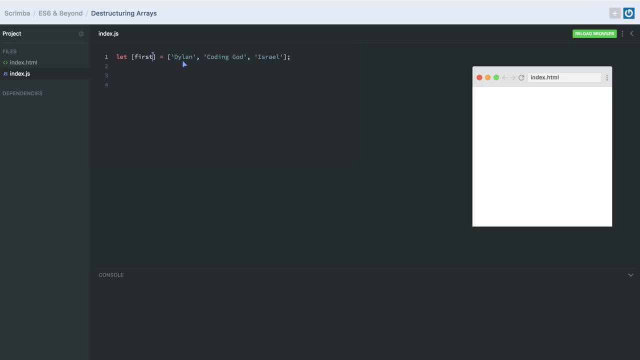 How might we do that? Well, we can go ahead and wrap it. Remember how we wrapped it with the object. We wrap it and we'll get first First name, like so, And we consolelog first name. You'll see, we'll say: we'll get Dylan right. 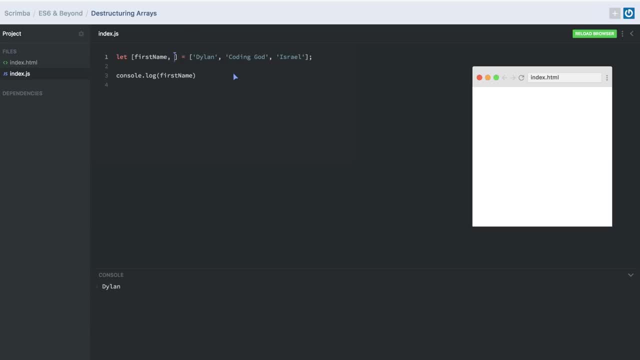 And then we can do multiple values right And we'll say middle name And we can pass middle name. We'll just do a little plus here and throw in middle name And it's going to not look very nice, but you'll see, we get Dylan Coding God or Dylan Coding without any space. 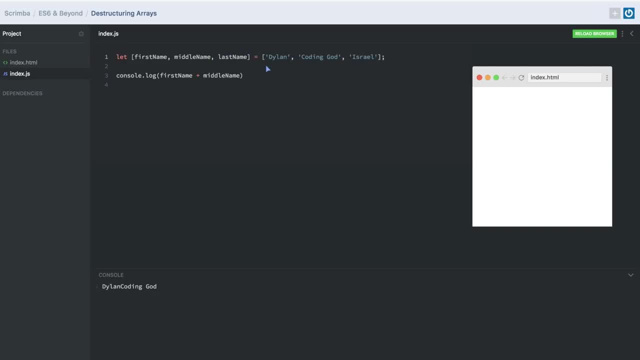 And we can do last name as well. But that's not it. Let's just go ahead and print this out piece by piece so we can see it's all working. Now you'll notice that it's going index by index. We don't have to have all of them, but we can. 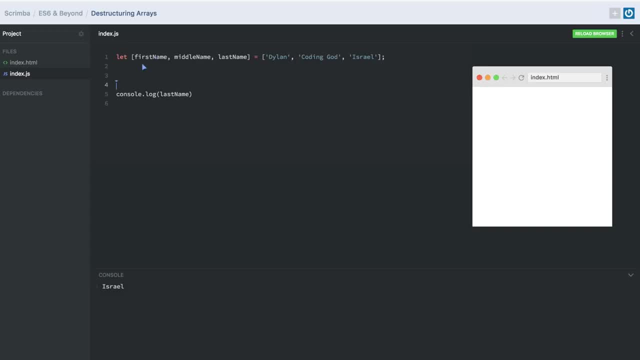 And in our instance we can actually reset the value here. So first name is actually storing a reference to that zero index. So if we wanted to overwrite the value in this case, we could, Let's say, I got a, let's go last name. 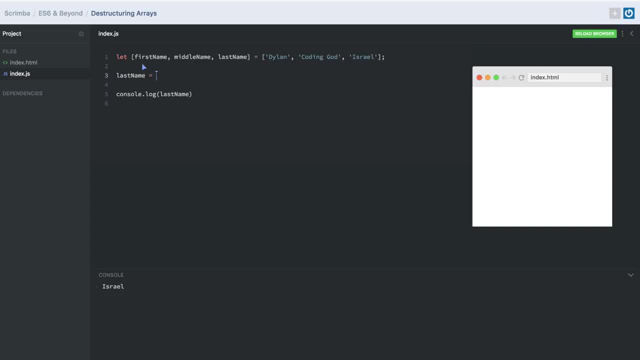 I got, let's say, my girlfriend I took, I took on her last name or something like that, And we just go ahead and I'll now become a Clemens. It's not going to happen, but we'll pretend Right, And now you'll see that last name becomes Clemens. 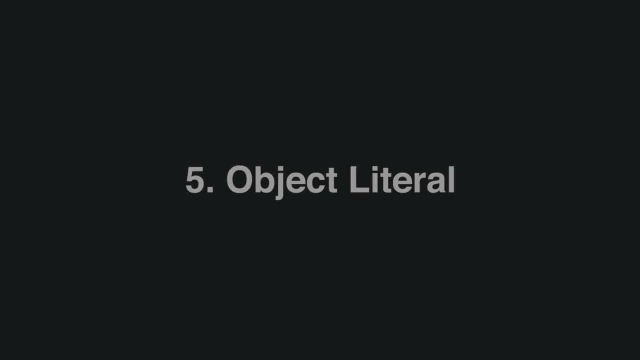 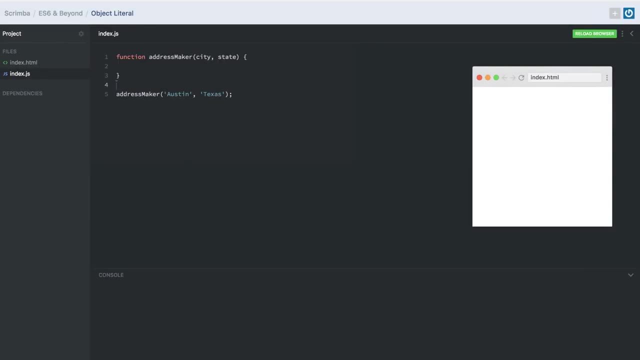 So this is one way that you can destructure an array. If you haven't noticed by now, ES6 has put an emphasis on writing less code while still being readable and maintainable, And object Literals are no different. So what are object literals? 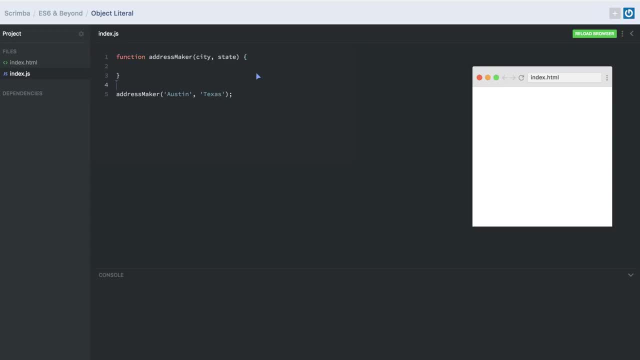 Well, a little bit of the setup. You see, we have this function here called address maker. It takes in two properties: city and state. Let's define a new variable and we'll just call this new address. Right now, we're going to set it to an empty object. 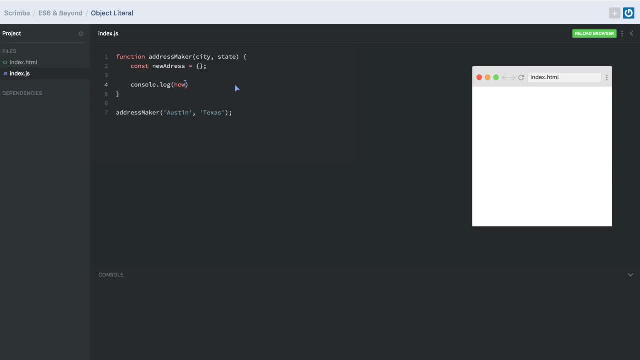 And all we want to do at the end here is: we're in console dot log new address. If we had, let's say, we'll have a property called new city And we'll set the value here to city, And then we'll have a new state and we'll set the value to state. 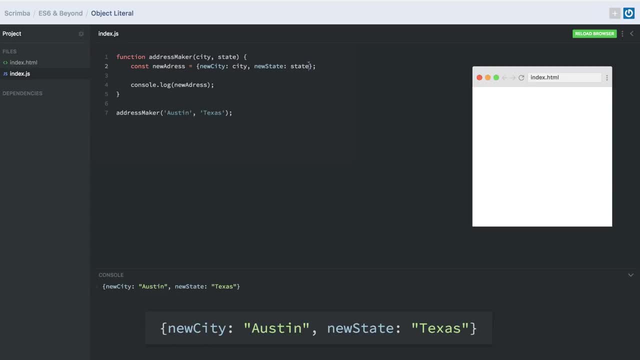 And then you'll notice that we print, print out. you know, new city, Austin, new state, Texas. as we would expect, Nothing new here, However, object literals give us the ability to, if these keys are the same as the value that they're passing in. 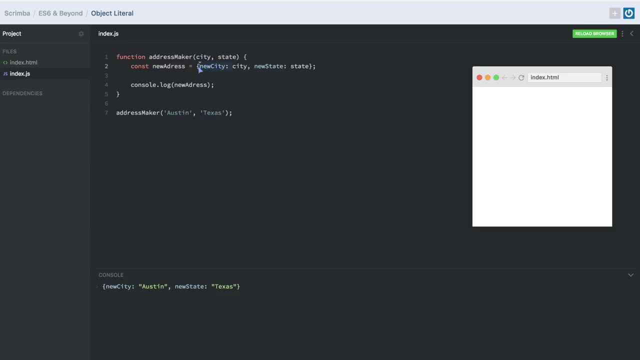 We don't actually have to set it. It's going to make the assumption. So in this case, let's say: instead of new city, the key was City. instead of new state, the key was state. What's going to happen here is it's going to assign the value of city to city and of state to state. 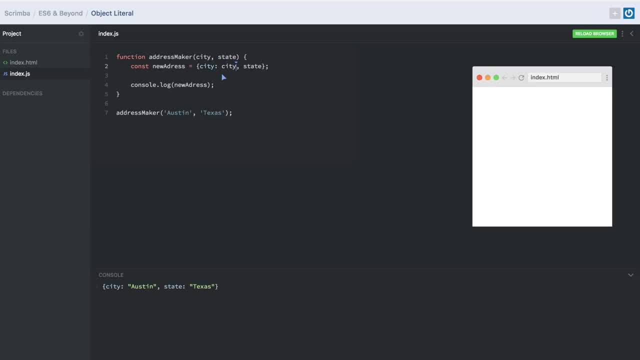 And we don't actually have to write: city is equal to city and state is equal to state, as you might have done in the past And you'll you'll see it'll work the same, But object literals give us the ability to do that now. 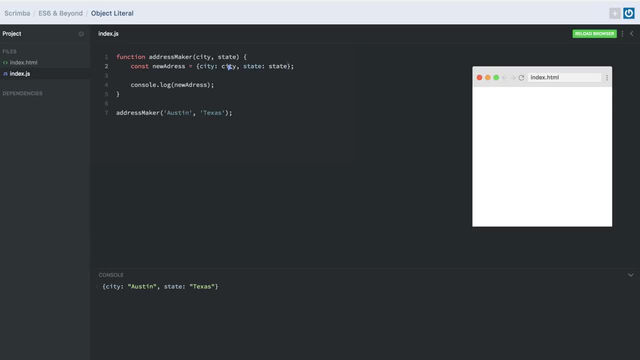 One caveat to that is, if you, If you are going to use object literals, just make sure it makes sense. Don't try to change your object or change your properties so much so that it doesn't make sense. But object literals is an excellent way for us not to have to write duplicate code. that doesn't help in explaining it but allows us to write less code while still being very descriptive. 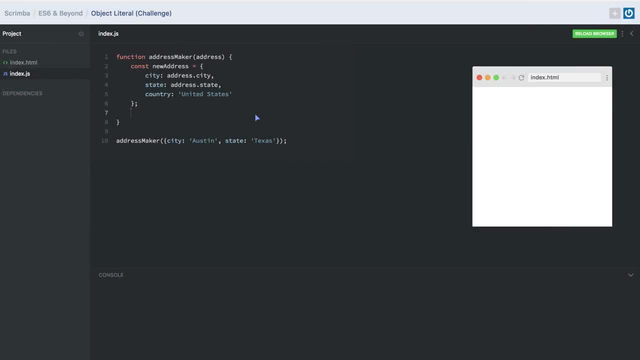 All right, In this challenge we're going to try and combine the template literal, the object literal And the object destructuring. How might we do this with the setup that we have here? You'll see, we have this address maker function taking in a city and state key in the object. 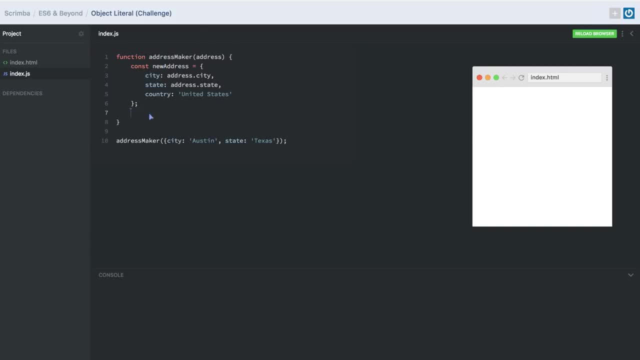 We then have this new address where we're applying the values that we're passing in And, on the end goal, all we wanted to do is console log the new city, the new state and the country with it, And we're going to use destructuring. 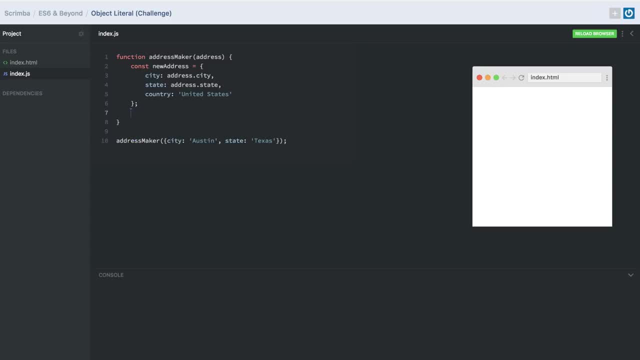 We're going to use template literals and we're going to use object literals. All right, I hope you took a second to try and figure this out on your own. If not, that's OK, And if you struggled, that's fine. 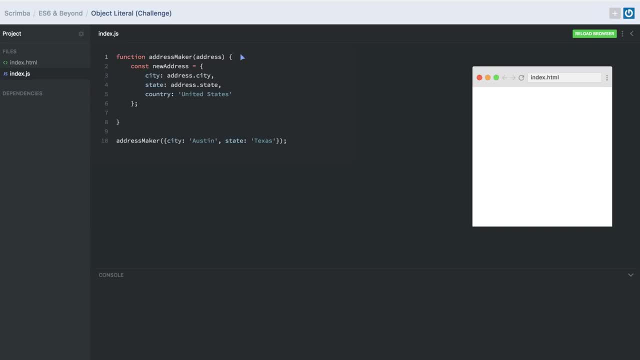 We're going to go through it right now. So what we're going to do here is we're going to create a constant and we're going to destructure our object. We're going to pass in the city, We're going to pass in the state. 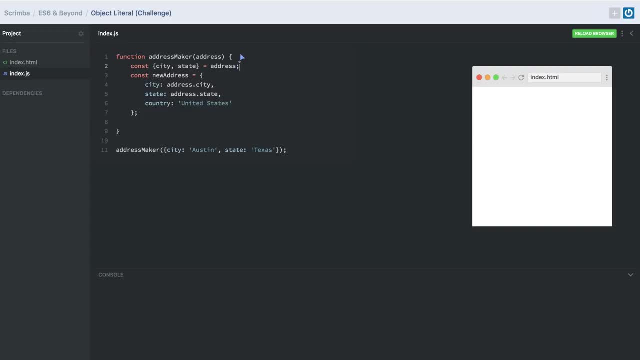 And we're going to set the reference to the address object that we're passing in. This is going to give us the ability to no longer need to say address dot city. We could, in theory, say city, city, but that wouldn't use the object literal. 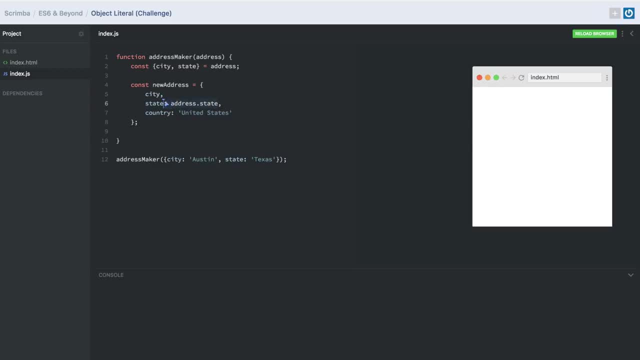 And so what we're going to do is we're going to get rid of the city. We're going to do the same thing with state as well, or the assignment of city, because this is going to know to say hey for the city key, assign this city value. 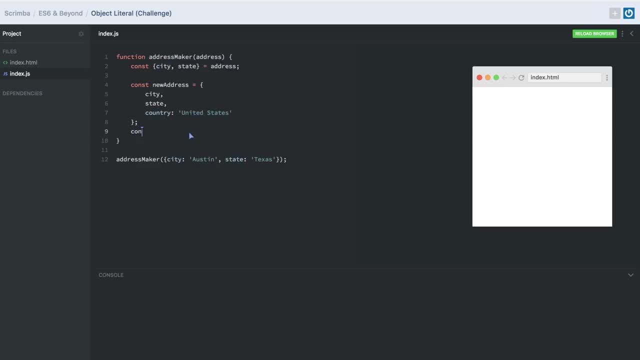 Then we're going to leave country alone. And, last but not least, we're just going to console dot log our new address using interpolation or template literals And we're going to say new address, city, space or comma, And it'll say new. 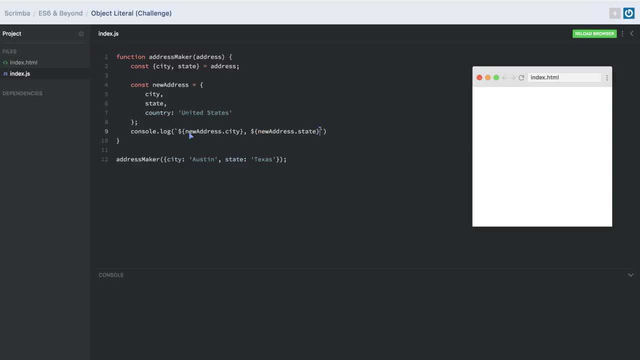 Address dot state. And then finally a little one more comma- And I'll do a last one here- of new address dot country. Save it And we're a good go. So you'll see: Austin, Texas, United States. The for of loop is a great addition to the JavaScript language. 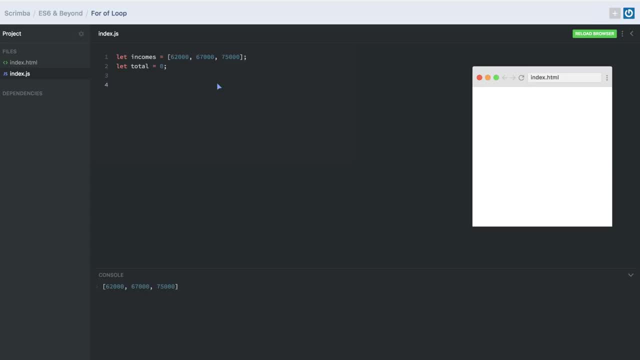 And let me showcase a little bit. So we're going to do a little bit of what it does say: we wanted to iterate over all these values in the array and perhaps add it to this total value, And at the end here all we wanted to do was console out, console log the total of the incomes. we could use the for of loop and it's going to start off as a simple for loop, and then we can define const. 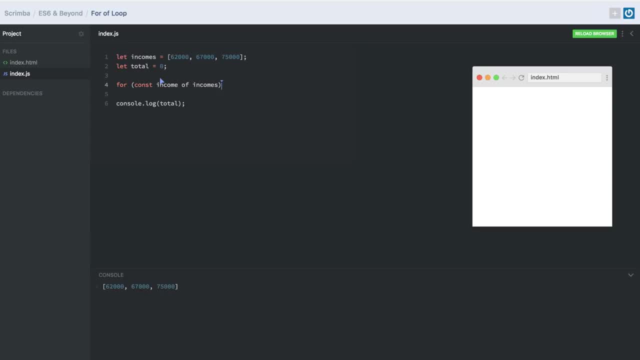 And we're going to say income of incomes And we're going to reset the value of anything in our logic nested in the for loop. So that's why we're using const. But if you're going to reset income nested in there and use it for some calculation or something like that, you would use let. 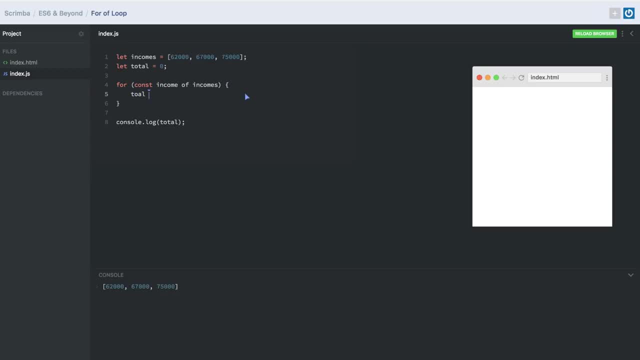 So we're going to say const And we're going to say total plus equals to the income we're passing in. We'll get something like 204,000.. Now let's check how we're. you know, if we wanted a console dot, log out income. 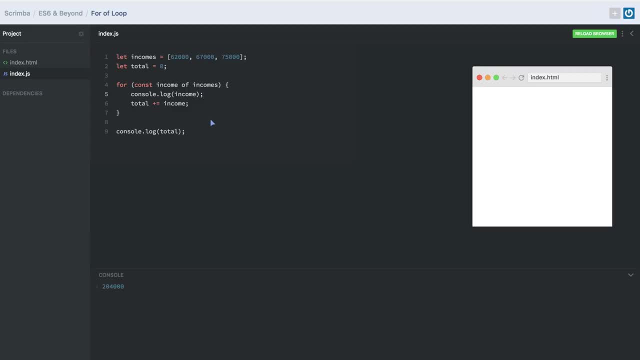 You can see we're going to get each individual income. Okay, get rid of that. So we get 62,000, 67,000, 65,000.. So this income here is saying each element in incomes or our iterable. 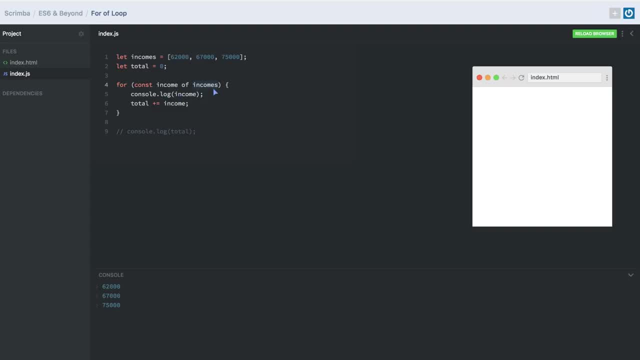 In this case, it's an array. We're able to do something with it, And so that's really what the for loop for of loop does is allows us to iterate through an entire, entire iterable. So you may have been wondering: why is Dylan? 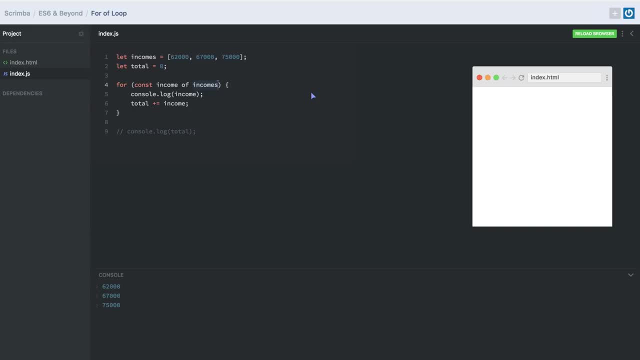 Keep saying. Why is he saying iterable and not array? Well, because we can actually use the for of loop with various iterables. What is another example of a popular iterable? Let's start off by get rid of our previous logic here, because they're no longer going to use total. 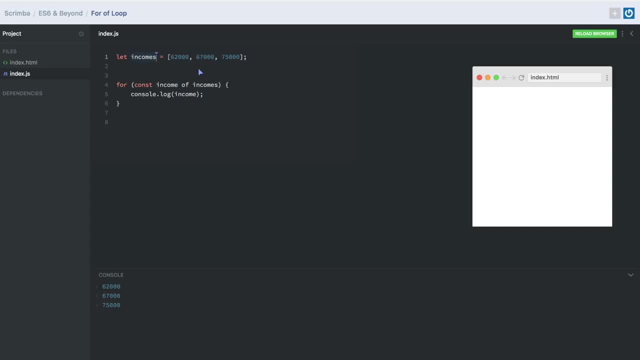 And we're going to change incomes to, let's say, full name, And we're going to set this equal to a string, So you can actually iterate over each character of the string, Like so: and instead of incomes we'll pass in full name instead of income. here we want it to make sense. 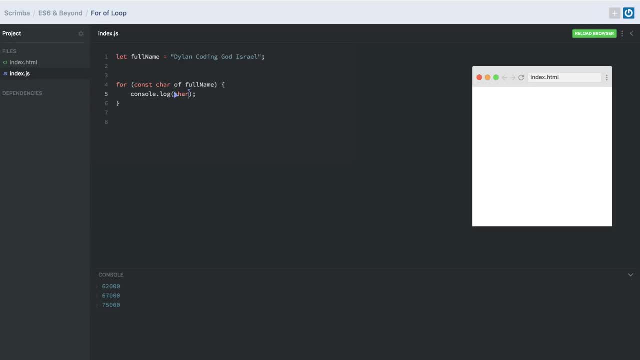 We'll just call it char and pass in char and we'll save it. And you'll see here that as we print out our logic, we get D Y L A N and then so on and so forth, And we can actually iterate over strings as well. 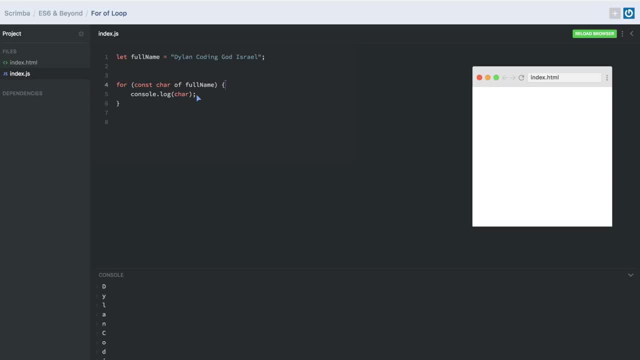 So anything that is an iterable we have the ability to go through. So that's map sets, typed arrays- And we're not going to dive into This in this course. perhaps later on we may do an advanced course where we break out all the craziness that you can do in JavaScript and some of the newer, newer types. 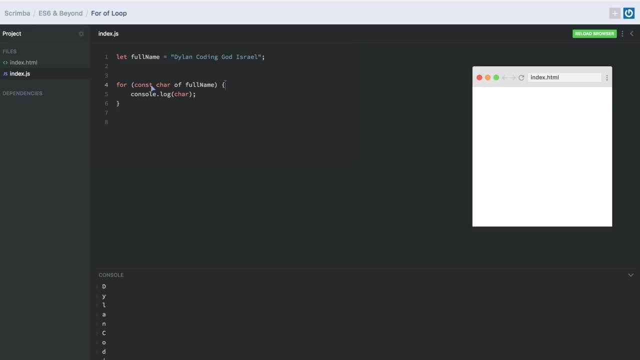 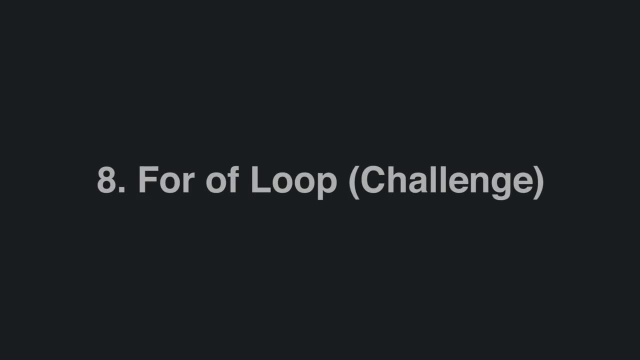 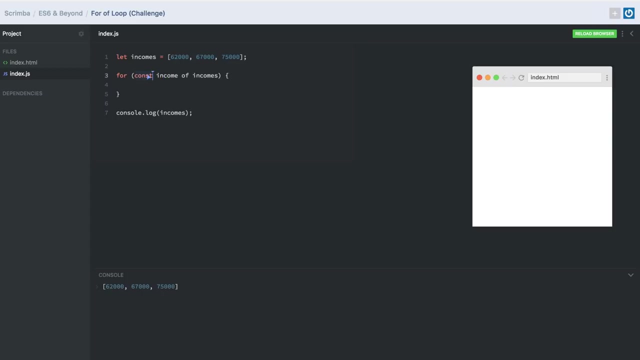 But here you can see that anything that's an interval we can go through with the for of loop. In this challenge we're going to pose the question of what do you think would happen if we gave each one of these incomes a bump of $5,000 and change this cons? 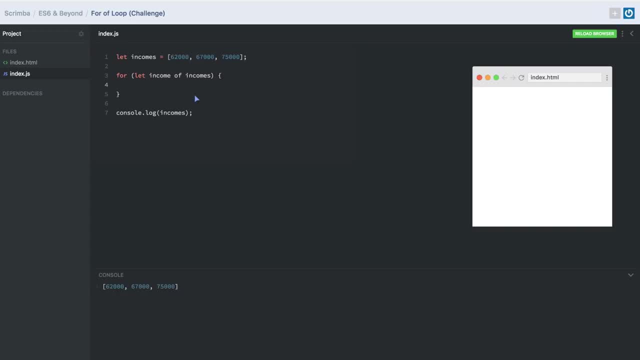 to a let and added $5,000 to the income. Would it change it, Would it not? Why might that be All right? So hopefully you took a second to figure out what this might be and just sort of think about it and let's see what happens. when we say, look, let excuse me, let take income and set it equal to itself and add $5,000. 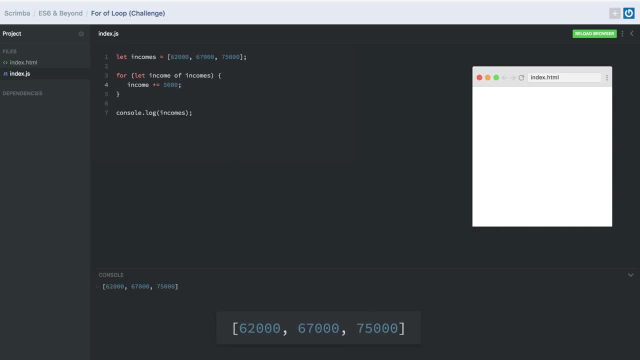 They all got a bonus. What are we going to get from incomes? You'll notice none of our values change. Well, we're using. the reason for this is: it's not. It's not designed to do that. You can, if you for some reason. we're going to add a value to this. 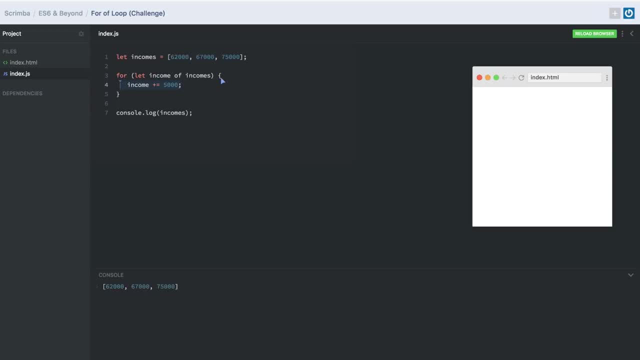 You don't want to create a new variable. You could do that and then store it elsewhere. But in this instance, when we're using the lead and we're trying to reset the value of the for of loop, that's not what it's designed for. 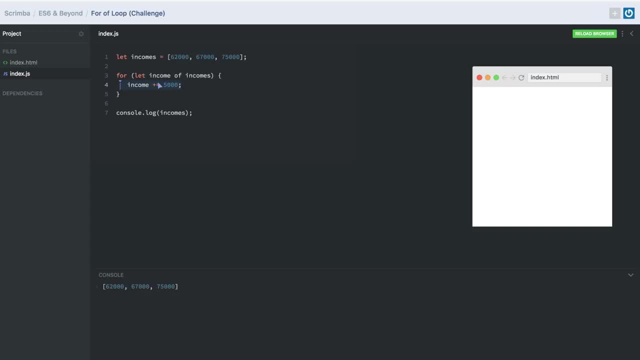 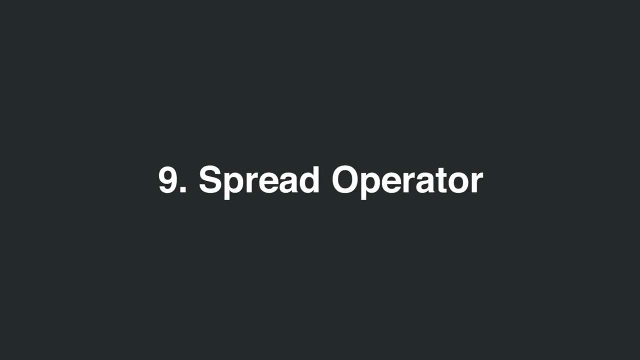 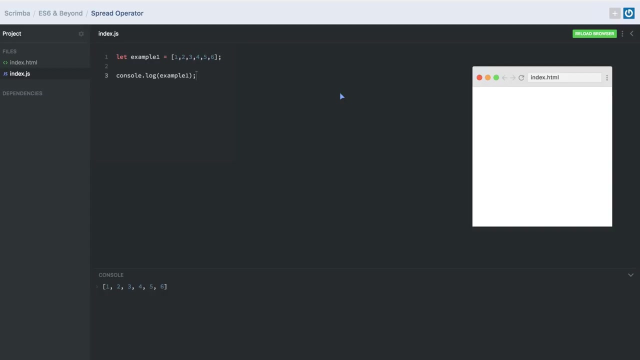 It's just designed to iterate over iterables, not actually used to set up new values or update the values of iterable objects. So what is the spread operator? This is another great addition to JavaScript, and one I use almost on a daily basis at work. 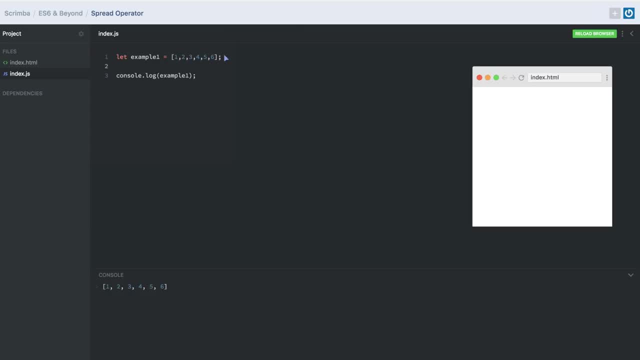 So the spread operator you'll see here in our, in our setup, is we have an array of values and then we're just printing out the values. Nothing special here. Let's go ahead and create this example two, and this is going to be an array, and then we're going to say dot, dot, dot. example one: 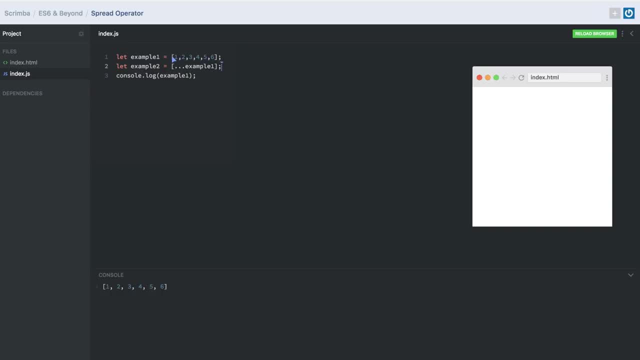 What is that doing? It's essentially Unwrapping the values of example one into example two and you'll see here, when we console log it out, all the new values are being added to example two, and it's also not passing it by reference. 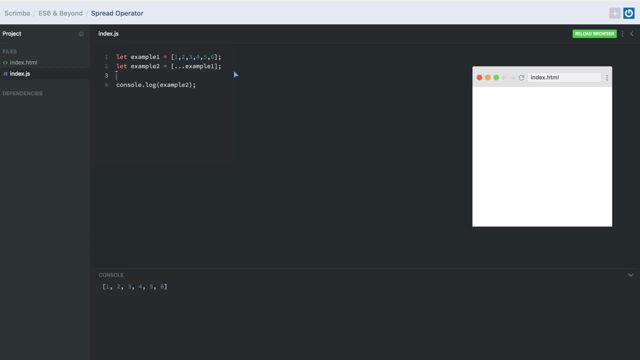 So is it instantiating a new array in this instance? And so if we were to take example two: dot, push a push. I want to just push a Boolean, Does that be a number? And then we want to check: hey, did this actually pass this to example one, if it was by value. 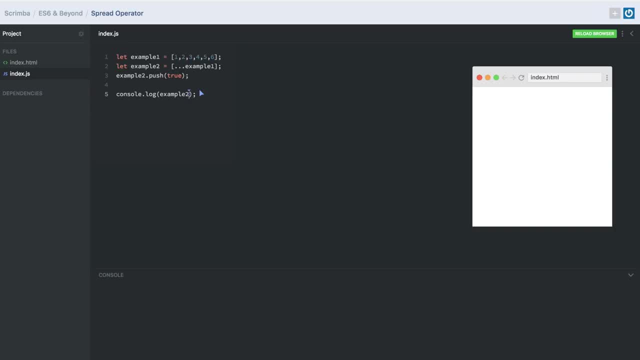 No, it didn't So, because we don't have that on example one there now the spread operator can be used with objects as well. Unfortunately, we're not going to be able to, at this time, showcase. I can show the an example of it, but we won't be able to actually see it in practice. 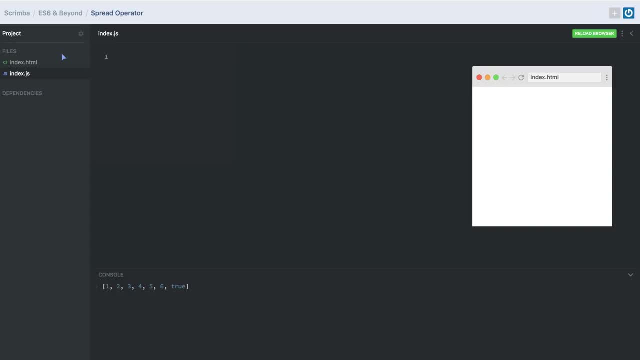 The spread operator when it comes to objects is a very new feature and something that the Babel settings that's running on Scriba don't currently compile, because they're probably a little bit more strict, as they should be. But an example of what might happen here is: let's say we have example one. 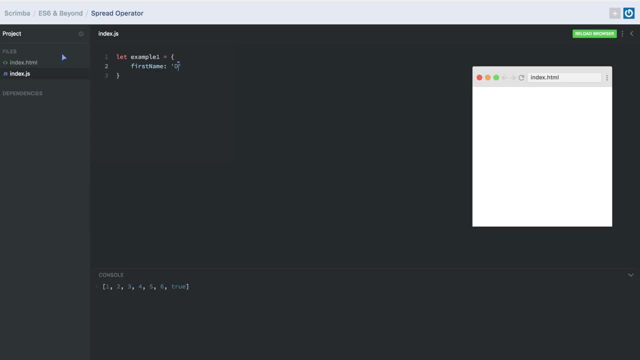 This is equal to an object of first name. So, Dylan, and then we said: let example two equal to an object, And then within here we might do dot, dot, dot. example one. And what would happen here if we were to- and we're going to come to this out because this isn't going to run- 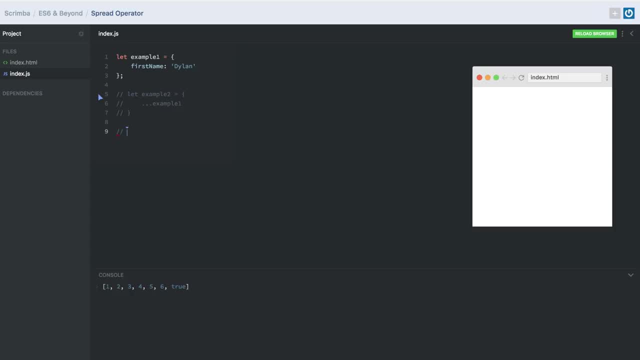 What would happen Here is that we would have our example to. Essentially, it would unwrap the keys and the values that are in example one and we get this object with first name, And with first name of Dylan. Now, there's a bunch of different reasons that you might do this. 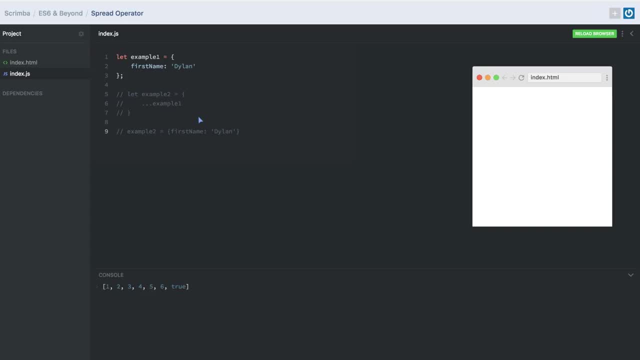 I do it in my constructors when it comes to TypeScript, where sometimes I'll have a default value. But when I'm doing this, I'm going to have a default value And then, for instance, I'm going to have a default value in case first name doesn't come from the back end. 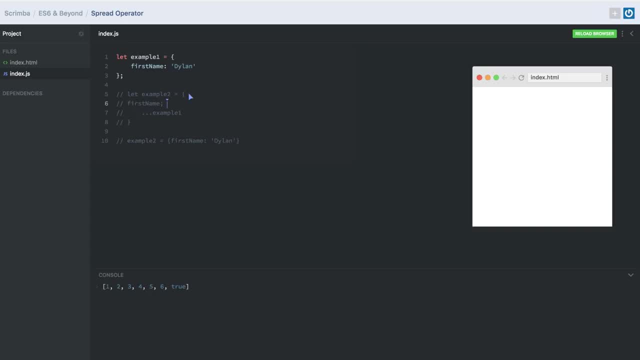 So I might have something like: first name is going to be equal to not applicable And that way when I'm writing my code is if something's not passed from the back end by need to have a value. Another great example is an empty array, because that will break our code if we're iterating over something. 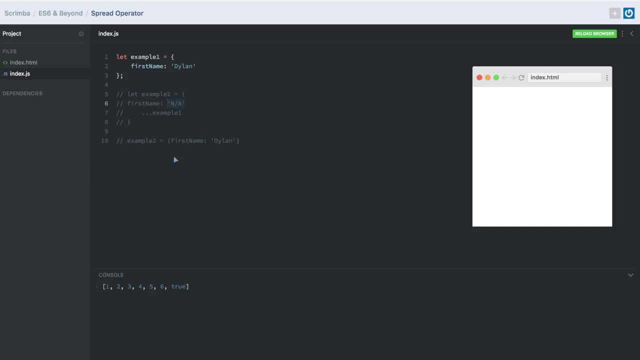 I'll assign an empty array unless something comes fulfilling that in the back end. So that's just one way of how you might use the spread operator when it comes to objects. So that's just one way of how you might use the spread operator when it comes to objects. 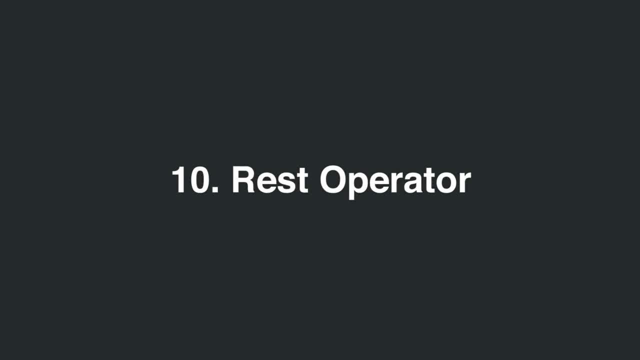 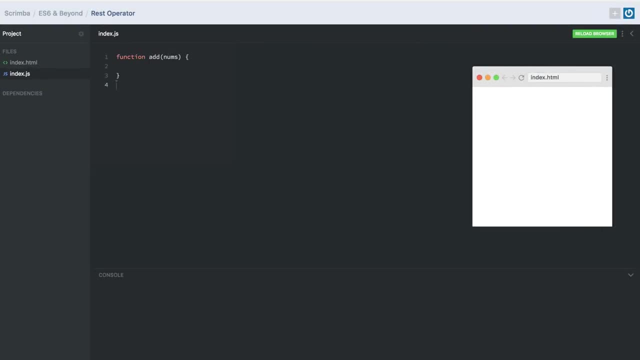 once it's a little bit more widely supported. The rest operator, although not as widely used as the spread operator, is somewhat similar and just as valuable. So what is the rest operator? It gives us the ability to get the arguments out of our function. 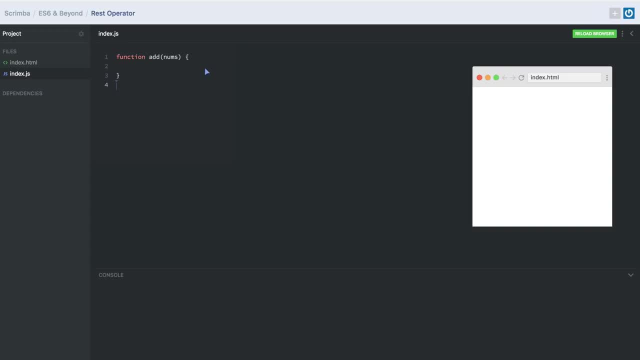 and it's used in a case in which we don't know how many inputs are going to be used. So in our example here we have a function add with a parameter called nums, And all we want to really do at the end of the day is consolelog nums. 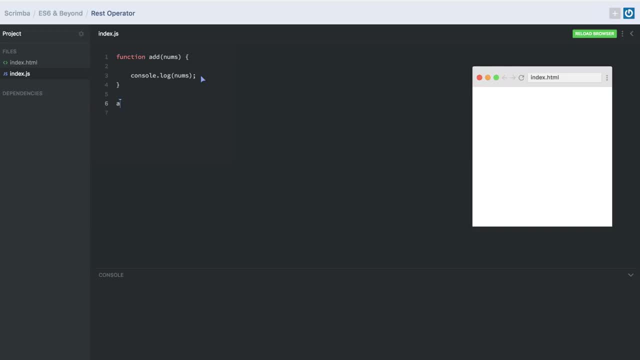 Let's go ahead and just add a function call real quick. So we'll take, add, We'll pass in 5 or 4.. And cool, it prints out 4.. What if we wanted this to take in as many numbers as possible? 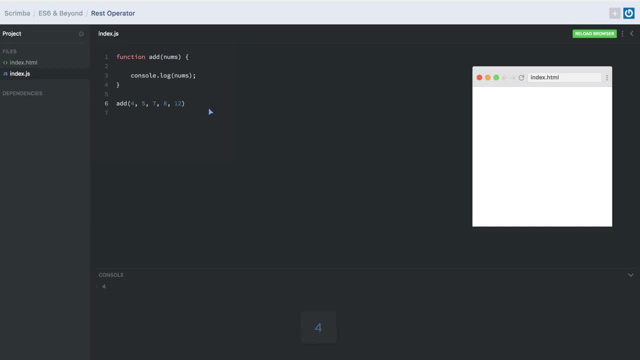 What's going to happen right now is our code is not going to do what we want it to do. We want it to print out all of nums And in the past, what we might have to do to get those out is we're going to print out all of nums. 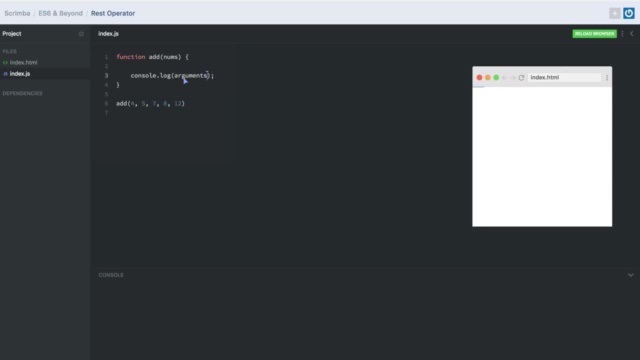 And in the past, what we might have to do to get those out is we're going to print out all of nums. And what we're going to do is we're going to print out all of nums is there's an arguments object for variables. 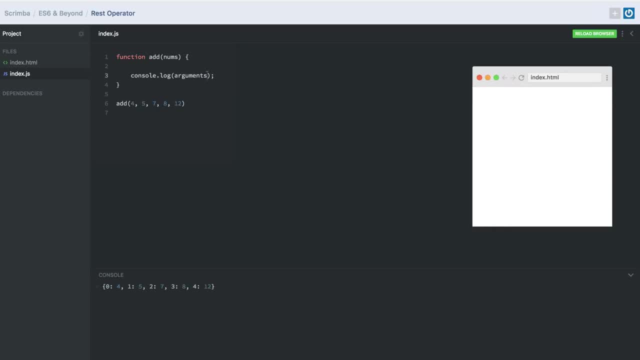 And you can see here it's actually going to say: look, this is on the 0 index of our add function. If you want to think of it that way: 0 input, then the 1 input and then we can get the values that way. 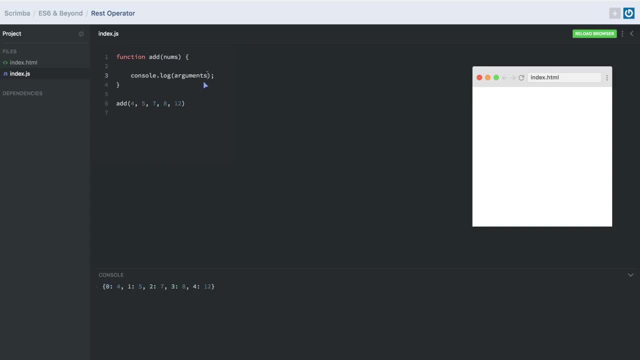 And we can do something with that. Now it's not an array, It's not iterable And typically that's what you're going to want to use. So in theory, arguments have sort of been deprecated unofficially with the rest. operator. 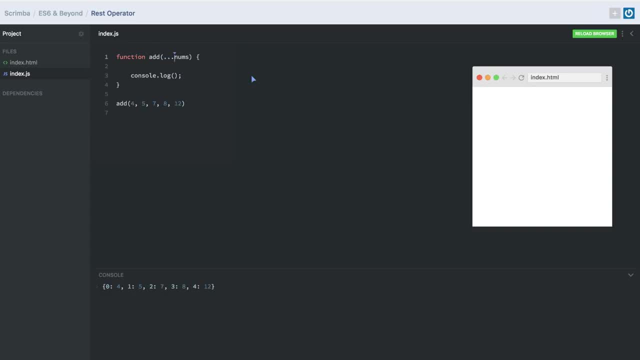 And what this is going to allow us to do is in our input here on the nums, you'll see we have the three dots. That's why I kind of say it's related to the spread operator. And now when we access nums, 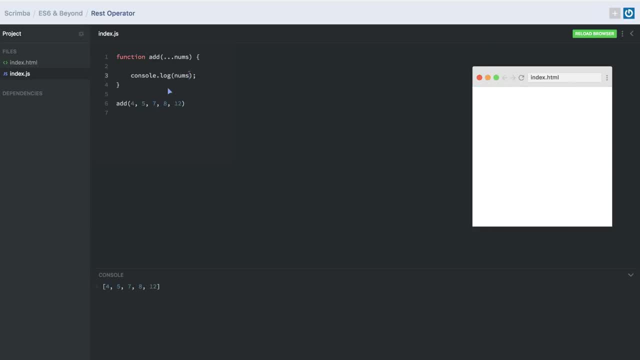 you'll see that we're going to get an array of the input values here. So when you're going to write a function and you don't know how many values are going to be inputted, you just know it's going to be some sort of value. 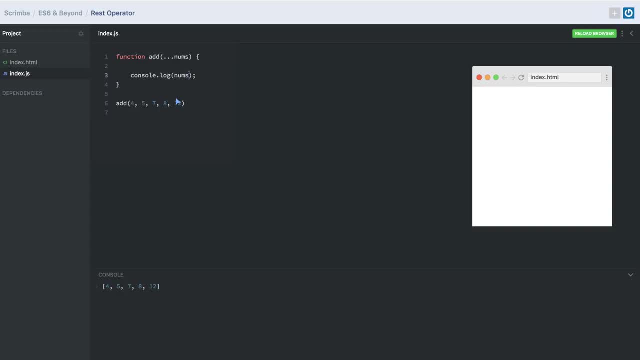 and you don't necessarily want to just pass an array, for various reasons, you may want to consider using the rest operator. It's extremely powerful. I use it whenever I need to. I don't use it as much. I use it as much as the spread operator. 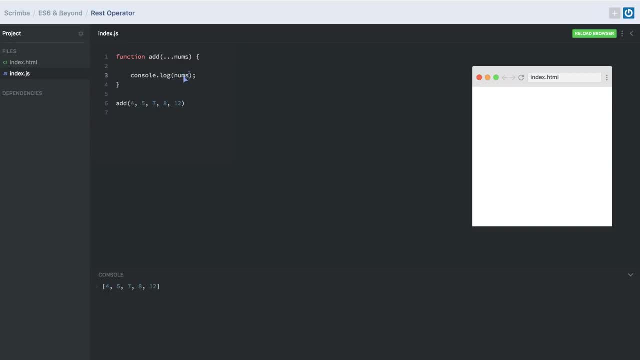 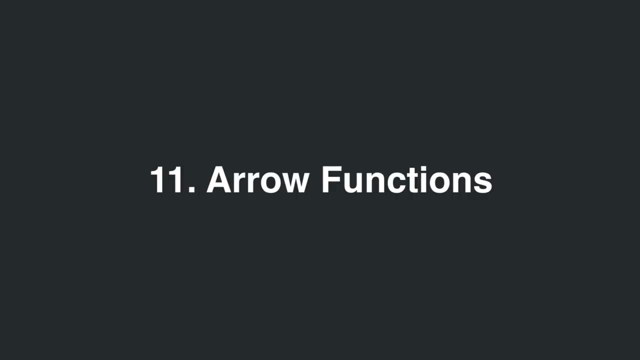 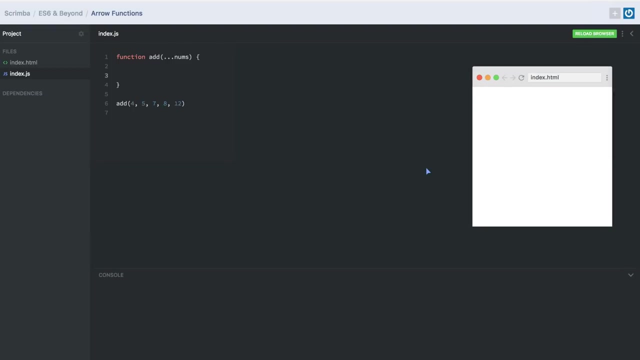 but I find it much more intuitive than having to convert the arguments to an array and get the values that way. So the rest operator is a great addition to ES6.. We're going to recycle a little bit of our code from the rest operator section. 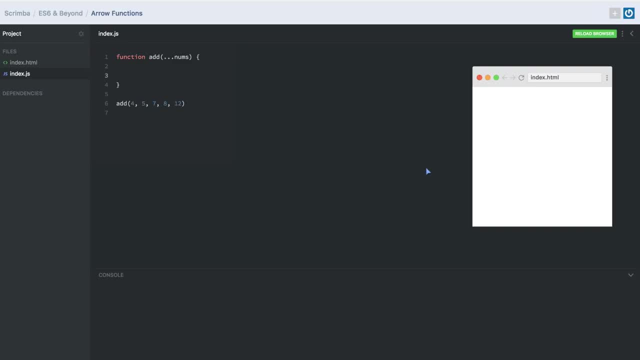 So just a reminder, here we have our function add that's taking in a numerous amount of values, And using the rest operator we're going to get an array of these values. Arrow functions are a great way to eliminate some of the really unnecessary boilerplate. 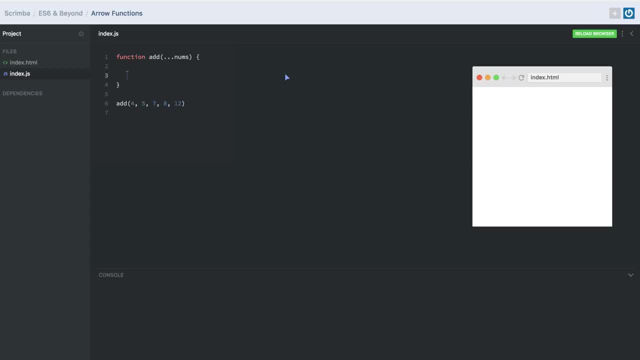 of callback functions And it comes with a lot of functionality, as well as such some gotchas that, if you don't know, exist. But let's start off by creating this total And we're going to essentially call the reduce array method, using arrow functions to return these values. 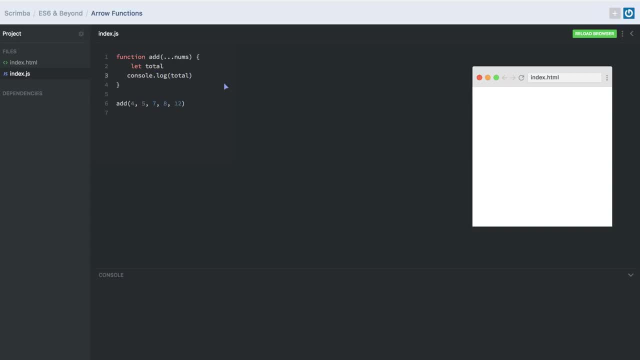 And then just below it we're going to say console dot log out total. Now, just as a reminder, nums- here is an array, So we have access to all the things that would come in it. So we'll have reduce And we'll just do x and y. 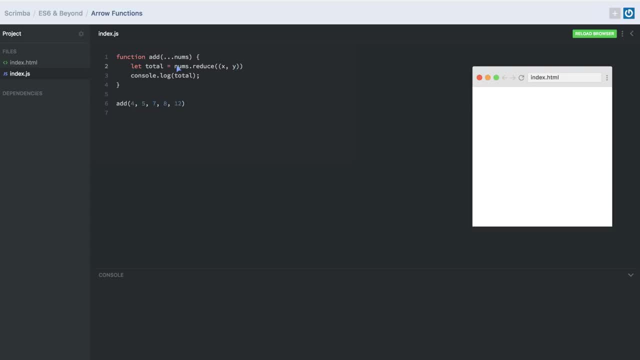 And you'll notice here that I've already by pure instinct typed this out. I wanted to show an instance of what we might do in the past without arrow functions, So you'll see function and then we'll define this with the brackets. 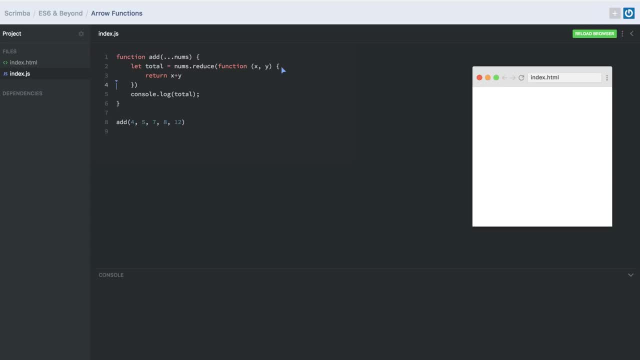 And then we'll say: return x plus y And then semicolon, semicolon, Go ahead and save, And you'll see we end up with 36, as it adds all the numbers together. So this callback function we can replace using arrow functions. 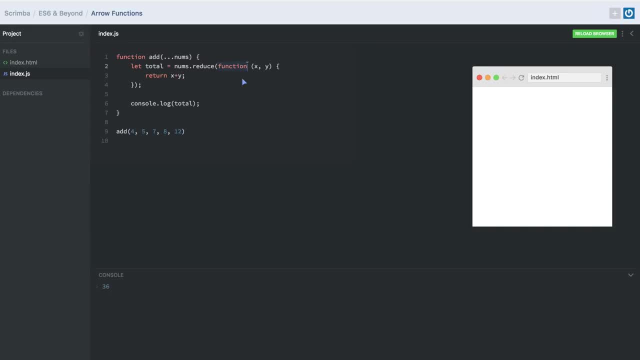 And the only downside to that is that it doesn't have its own instance of this, which may or may hurt you in your code. So if you come across that, really just be aware that that is part of the trade-off for what we're doing here. 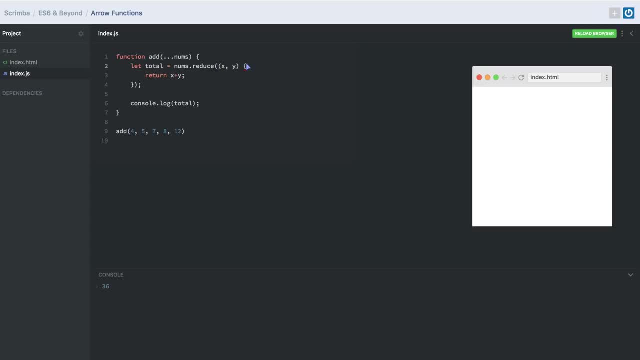 So let's go eliminate this function, And so we can eliminate this code. And you're saying: well, why are we in this error? Well, when we eliminate function, we have to assign this arrow function, hence the name. You'll see it still works. 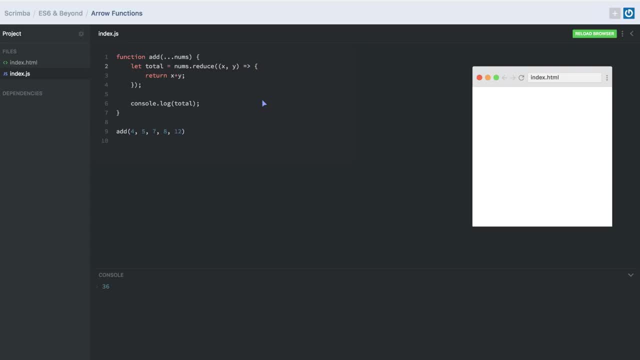 But we can actually eliminate even more code at this point where, if we're doing a simple one-line return in our arrow function, such as just adding these values together, we can eliminate this curly brace here And we can also eliminate this return statement. 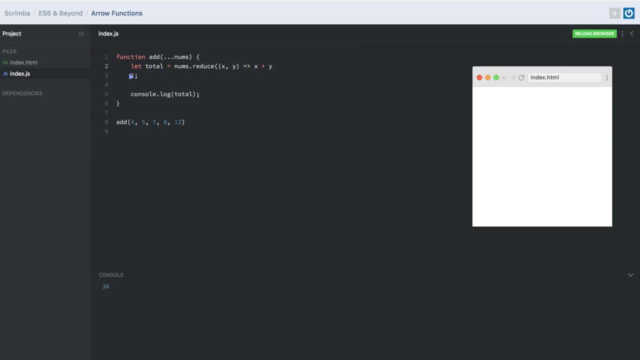 And we can eliminate this semicolon And what we get is a very clean arrow function that will return the values that we're looking for, And we've eliminated maybe 20 characters of code and a lot of spacing for something that we really didn't need to get going. 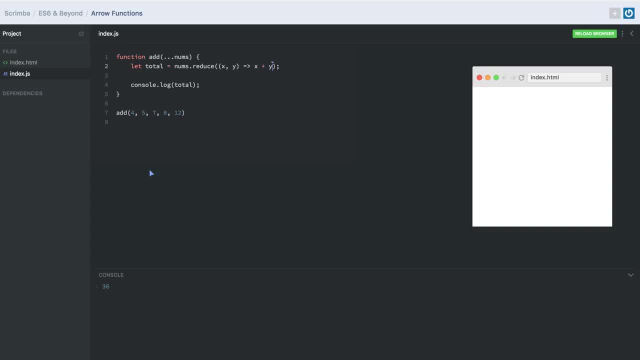 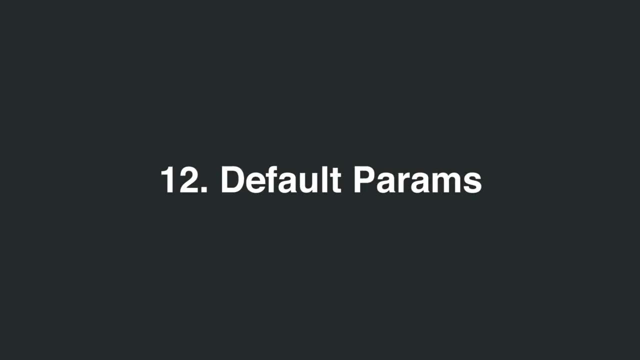 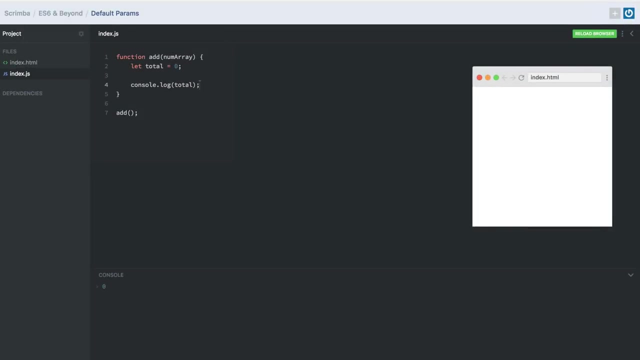 So arrow functions are very powerful And they're also just very condensing. condense and eliminate a lot of the useless boilerplate when it comes to callback functions. Default parameters for JavaScript is another new concept, but it's been around in other programming languages. 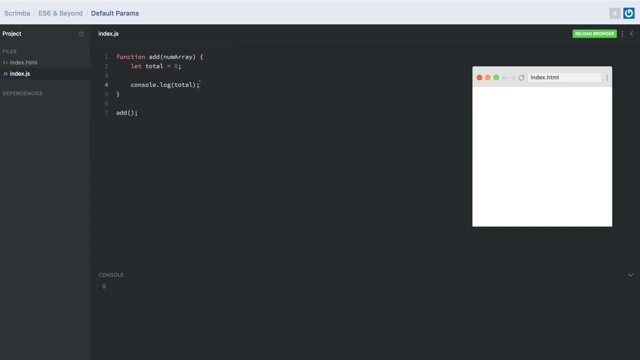 for quite some time And it provides us a lot of value. that's going to stop a lot of forced error checking and forced error prevention. And let's take a look at our code here. where we have an add function, It takes in an array presumably. 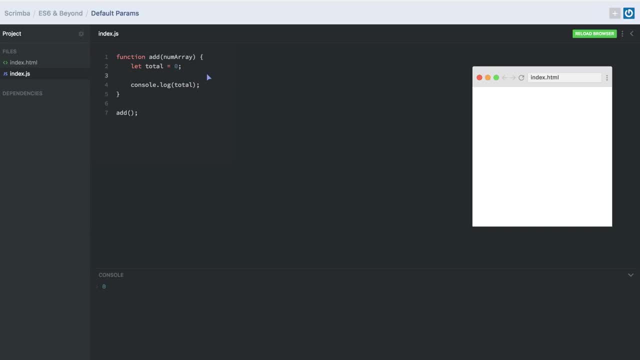 It's called numArray And you'll see here in our add we're not calling it, which right now we're not using numArray. But let's say we were. We wanted to, for each iteration of numArray, run a foreach on it, take an element. 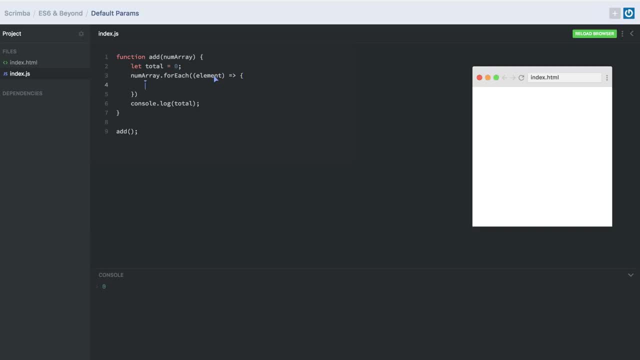 You'll notice. we're going to go ahead and use the arrow functions And we want to say total plus equals to that element. What's going to happen here in our current iteration is we're going to get an error right. Type error for each of undefined. 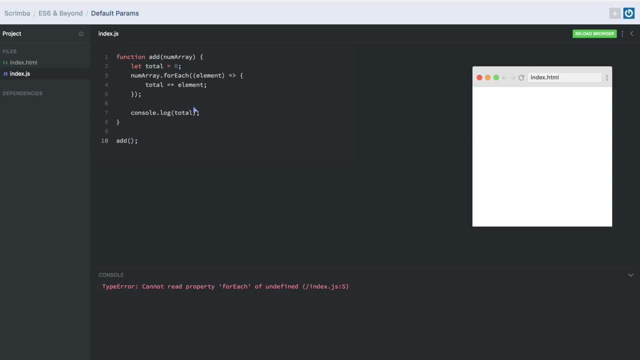 We never pass in numArray, That's going to give us an issue because we don't have an array to iterate over Now. what we can do instead is we can use optional parameters to help prevent this from airing our code out, Because sometimes maybe someone calls it. 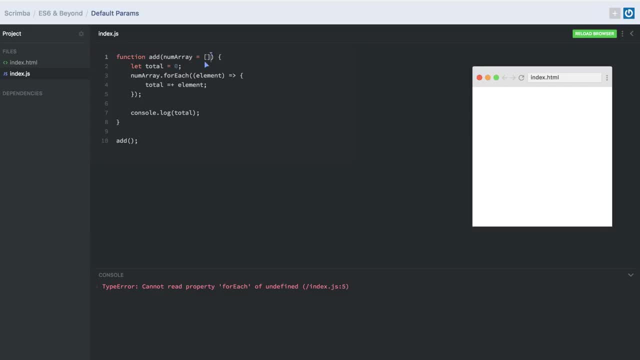 Sometimes maybe it doesn't matter, Sometimes it's just going to be an empty array or whatever the case may be. But now what happens is, when numArray isn't passed in, we are providing an empty array, saying hey, if it doesn't exist, set it to an empty array. 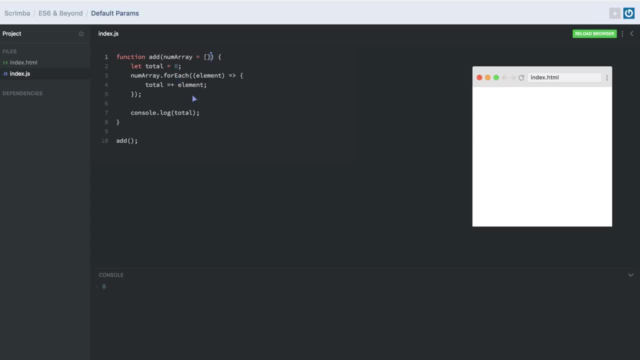 Therefore our array methods don't break, And then, in our case, we just get a total that returns zero, because there's nothing to iterate over, and thus nothing gets added to the total. So and plus equals. there we go, And thus we have a solution in place. 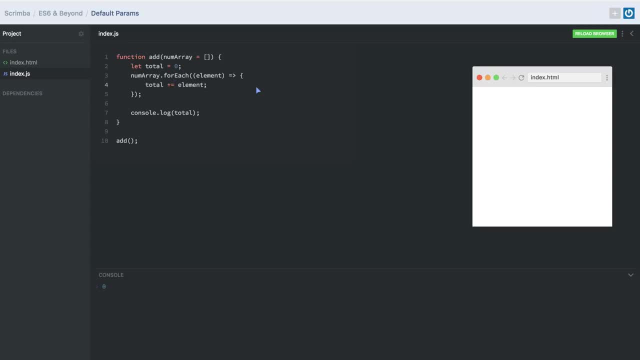 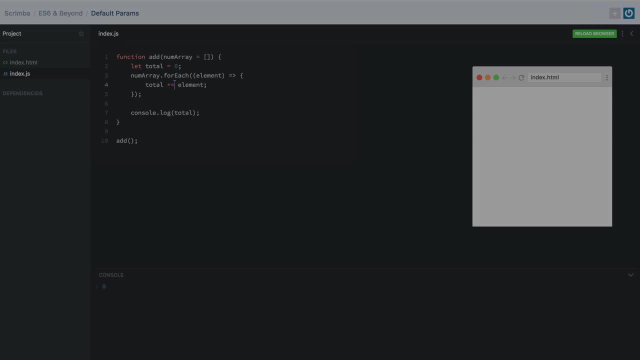 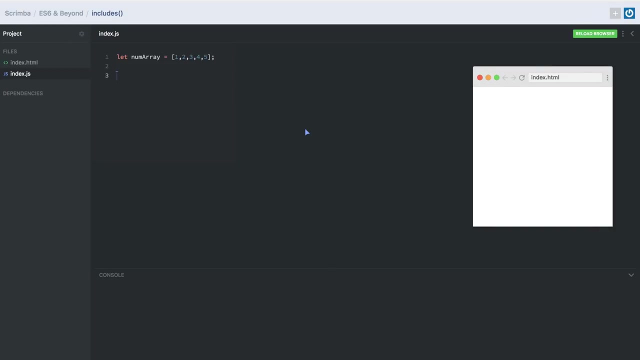 to prevent those undefined errors that will be so rampant, especially when you get incorrect data, maybe from APIs or the backend, or even just your own logic or user input. JavaScript's always been kind of a strange language in the fact that we don't always have a method. 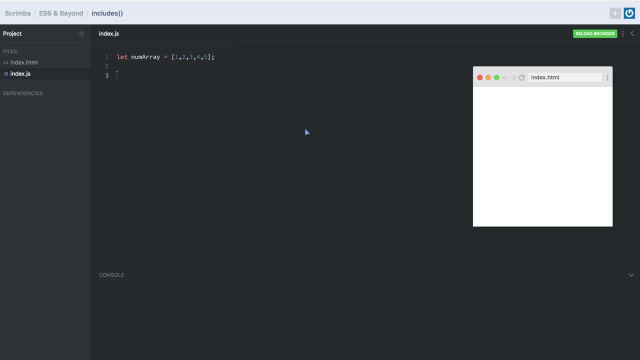 that does what you would expect a language to have, And so in the past when we wanted to check if an array had a value, we would use indexOf. So in our case we have consolelog and we say numArrayindexOf, And indexOf of course returns the index of values in there. 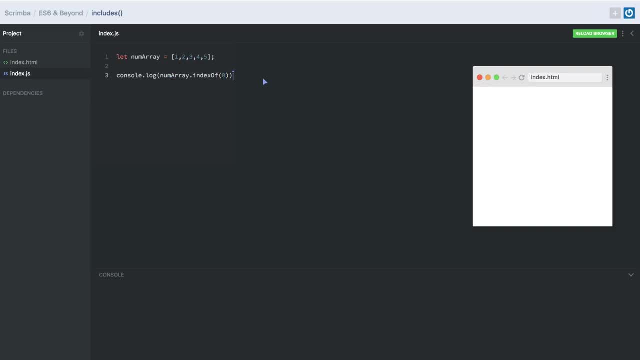 And if it's an index value like zero, it's going to return negative one because it doesn't exist. That's kind of wonky, And so we got introduced to a new method called includes, And includes will return a Boolean value of true or false. 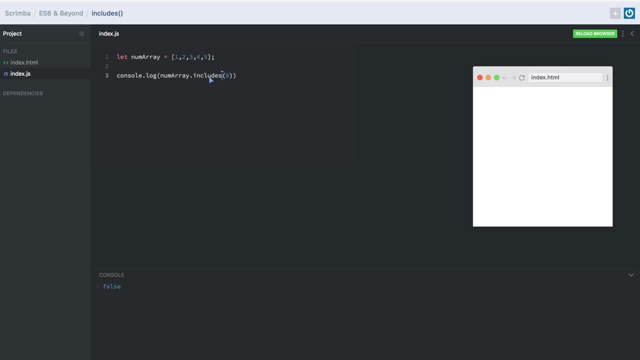 So you'll see, here, when we throw in zero, it's going to return false, And when we include two here, it's going to return true, because it's contained within the array. One thing to keep in mind for this: if you are trying to support, say. 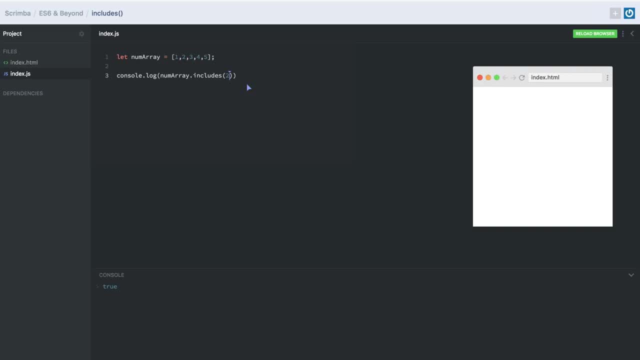 Internet Explorer. for some unknown reason, you may run into issues. This is not supported by Internet Explorer, but it is supported by all major web browsers besides IE. We're going to talk a little bit about let and const, but in order to understand why let exists, 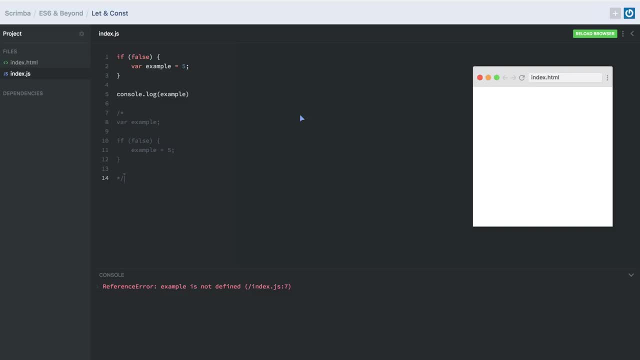 and const for that matter, exists, you have to sort of understand a variable hoisting in JavaScript. Let's take a look at our example code right here. You'll see that we have. if false var example is equal to five, consolelog example. 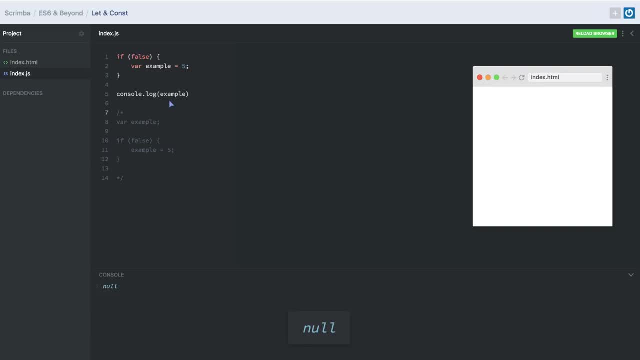 Now, what may surprise you is that we're going to get a null value and not a like. this is completely an error. Why would you log this value? And that's because of what's called variable hoisting when it comes to JavaScript's var. 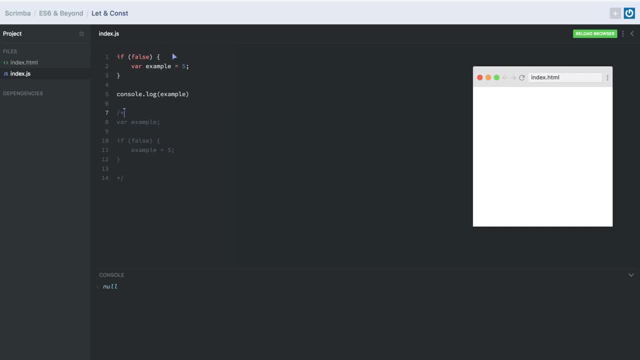 is it hoists the variables, And so what JavaScript actually sees when this renders is what's in our commented out code here is it hoists the var example and it hoists it to the root, essentially to the function scope level, And then it looks like: oh, example is equal to five. 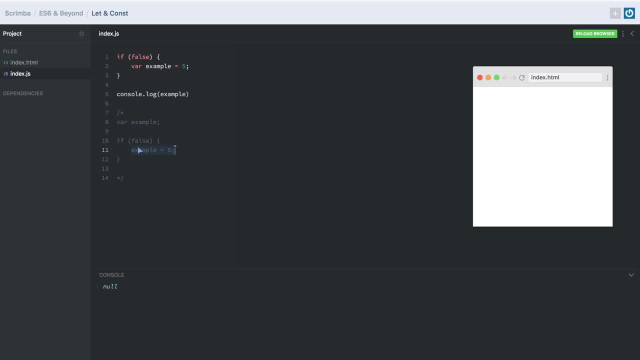 and then console logs it, So it hoists a variable And this is solved by using let and const. moving forward, So let's dive in a little bit about let and const. So let essentially is a stricter version of var, in which it uses block scope. 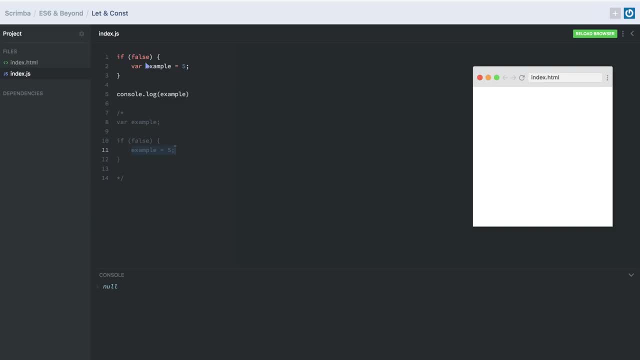 So in our case right now, we're getting a null. We're getting an error, though, when we try a log out example. However, if we go ahead and define let, in our instance here, you're going to see that we're going to get a undefined error. 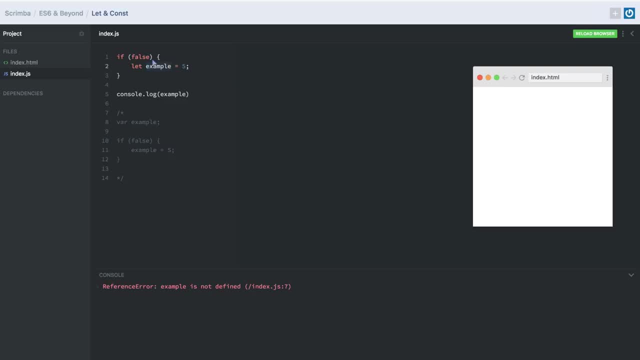 because the example variable doesn't exist unless it's within this nested block scope, as you might imagine, because the way that it's actually interpreting it is exactly how it is printed, which makes a lot of sense. So var is using hoisting, let does not. 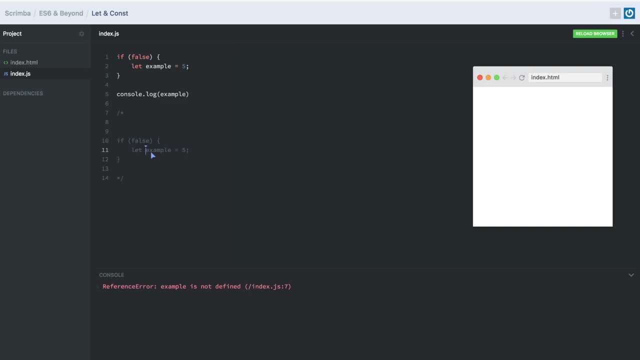 and neither does const And moving forward, you, for the most part, should be always using let when you're going to have values that are reassignable. Now let's dive in a little bit about const and how that differs from let. 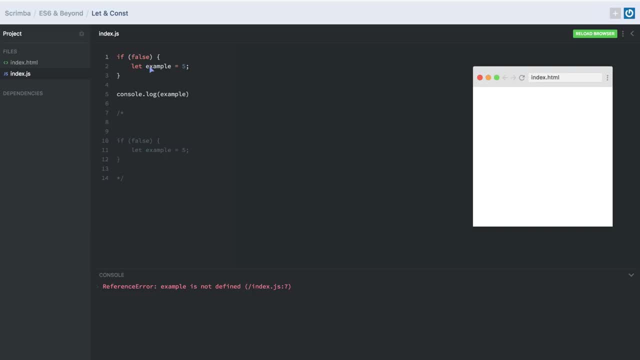 Const, as you might have guessed, stands for constant, but it may not work in the exact same way that you would expect, So let's go ahead and clean up our code a little bit here. Const is denoted by the const word. 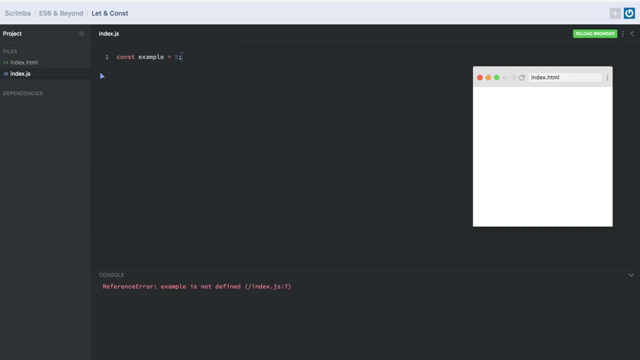 And we'll just say example, And we're going to set this equal to a primitive data type, which would be a number, a string or a Boolean, So we're excluding objects and arrays. Now, what you may see, constlog, as you would expect in our example. 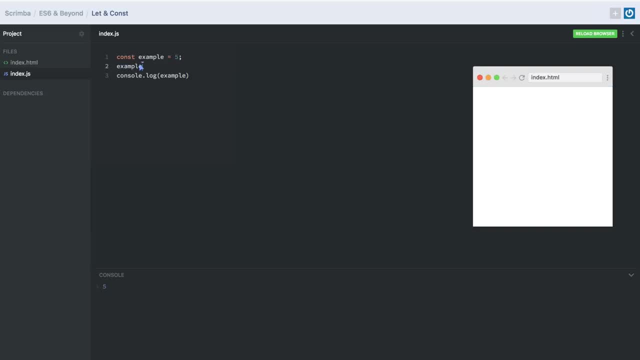 we're going to get the value. However, we can't actually reset the value. Example, when we're dealing with the primitive types will give us an error, So we'll set this to 10.. Doesn't matter if it's the same type. 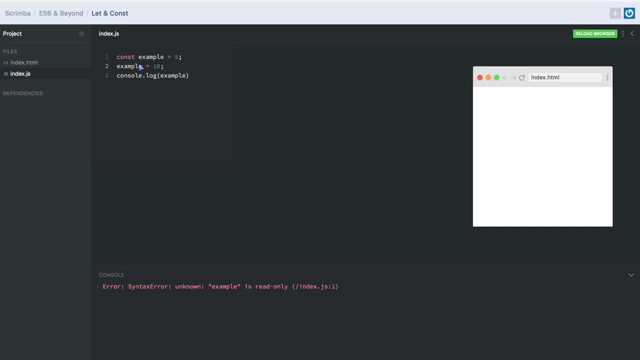 Example when dealing with the primitive types are read-only properties. These are things that have been set and you don't plan on changing. However, where this may get a little bit confusing is this: It's not necessarily the case when we're dealing with arrays. 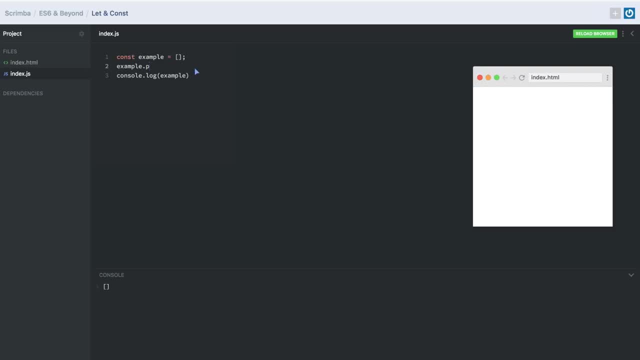 So in our case we have an empty array, We can actually still, in our const example, push to it and set it, you know, push a value to 5.. That's fine. However, if we wanted to change the value, 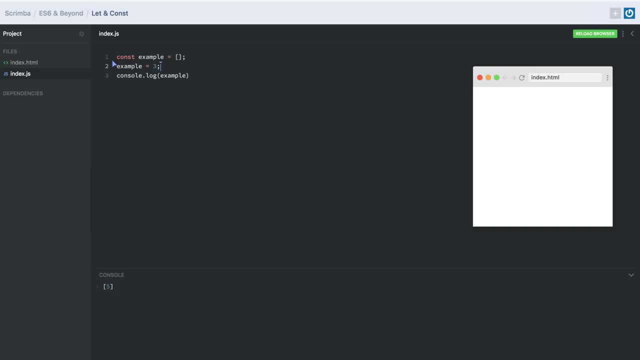 from an array to I don't know 3, we're going to get a syntax error. So that's not okay. And that goes the same for objects. If we have an empty object here and see empty object, we can actually assign properties to it as well. 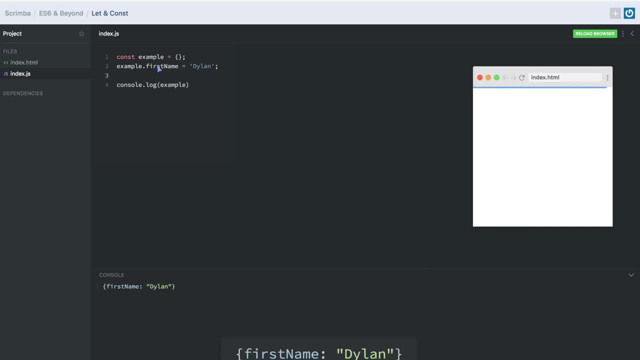 And this will work similar to how array works. So, although const is sort of a constant theory, it's not exactly. You can modify objects in arrays, but you cannot override the data types with those moving forward And when it comes to primitive values, 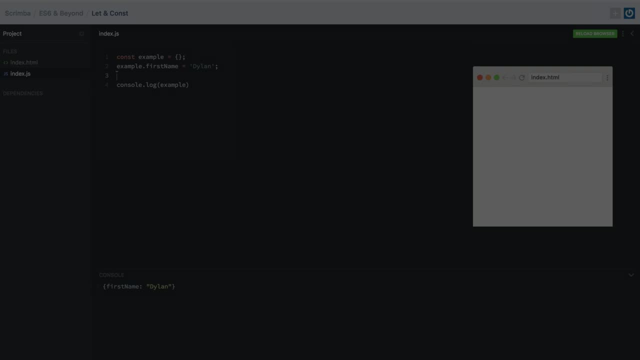 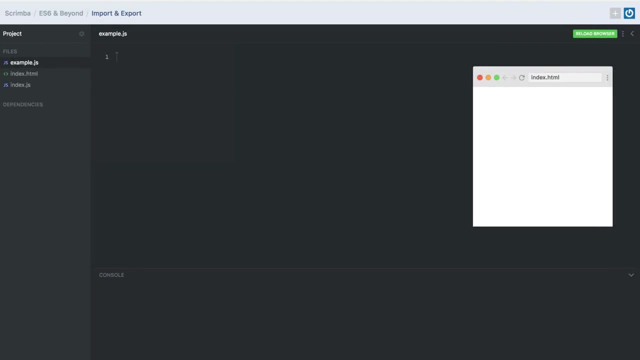 the numbers, the strings and the booleans. you can't change those at all. Import and export have been a great addition to JavaScript. It allows us to follow the solid principles and do dependency injection and more object-oriented programming and essentially allow our code to be more modular in nature. 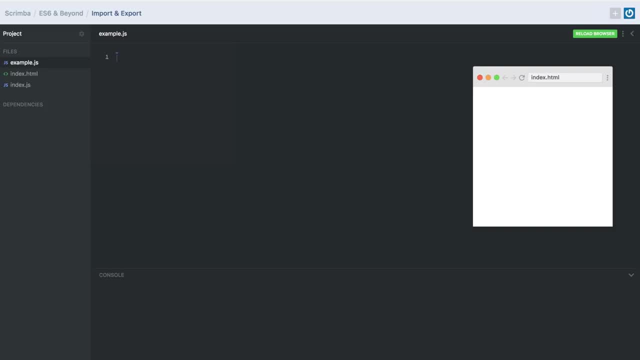 which lends it to be more easily organized, which is a great thing. How do they work? What do they do? Well, let's take our examplejs file that we have here and define- In this case, we're going to define just a variable. 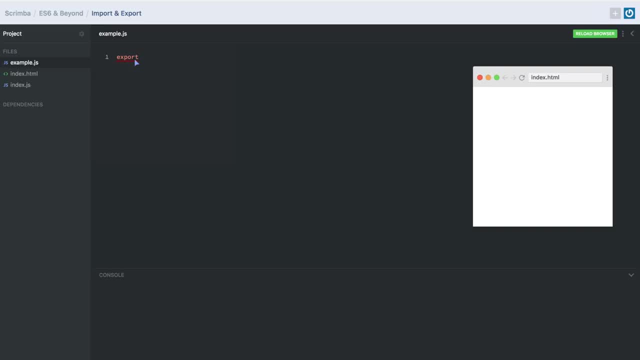 a const variable, And the reason that you might do something like that is you may have a data set that you're going to use by multiple parts of your application, or it may just be long, It's cleaner and you just want it in one spot. 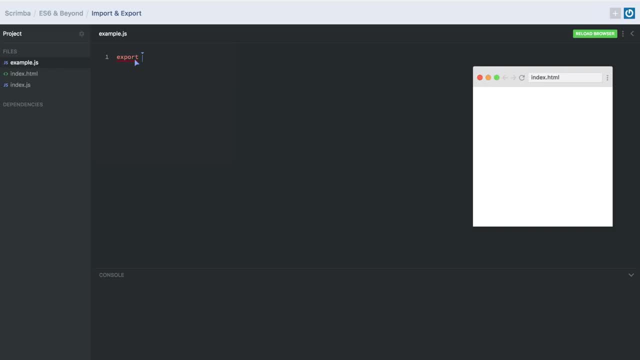 It really just doesn't matter. But in our case, here we're going to find a const and we're just going to call it data, We're going to set it equal to an array and we'll go ahead and throw in maybe a 1,, a 2, and a 3.. 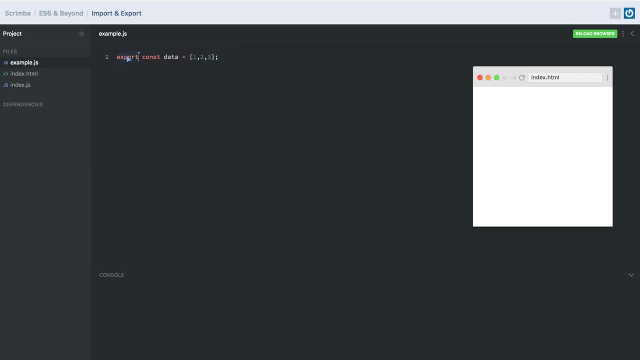 It doesn't really matter in this case. So this export allows us to, in this case, export data which we can then import in another application. You can do classes, You can do enums if you're working in TypeScript and stuff like that. 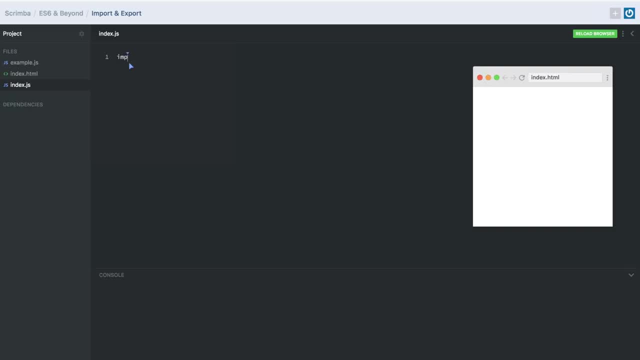 Let's go ahead and show how we can import it. So we'll have this import and then these two curly braces. Now remember how we had data here. That is what we're going to be importing within these curly braces And in our example here. 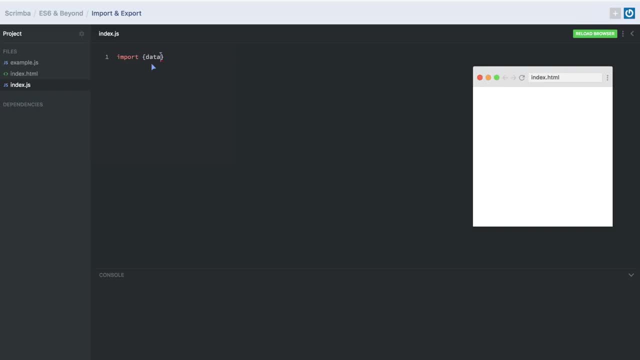 we don't have multiple things being exported, But if we did, like a data 2, you would just throw a comma and then you'd have access to it. We're going to import data and typically you want to space it out like so: 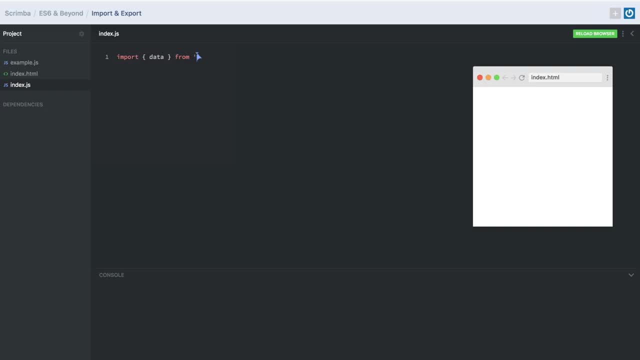 And then you have to say from where. In our case it's just from the examplejs file. And now if we wanted to consolelog data, we could, and you'll see, here we actually get our 1,, 2,, 3.. 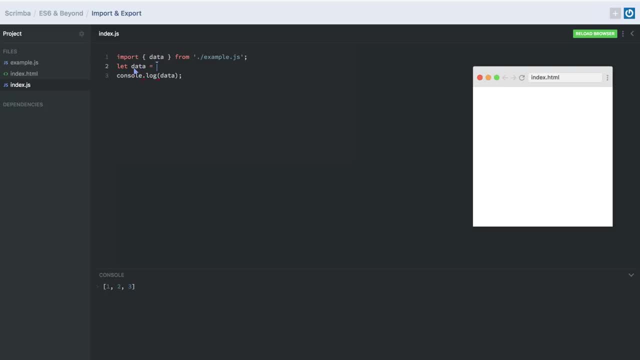 We'd even create a reference to it- let data equal, let updated data equal data- And then we could push to it if we wanted to as well, and just treat it like any other item that we wanted: Updated data. There we go. 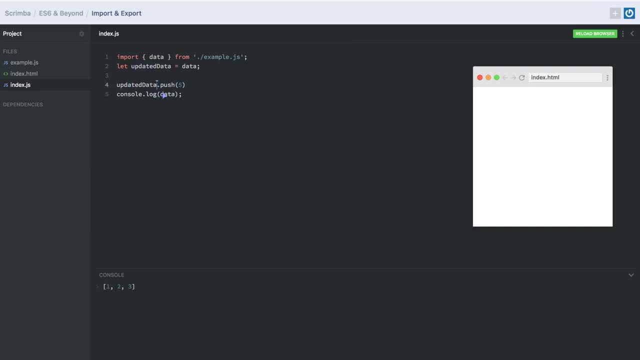 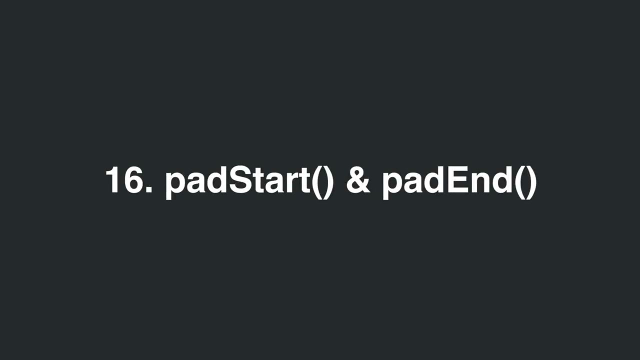 Oops, Updated data, And there we go. We get 1,, 2,, 3, and 5.. So this allows us to make our code more module, as well as be able to organize in such a way. It's very helpful and something I use on a daily basis. 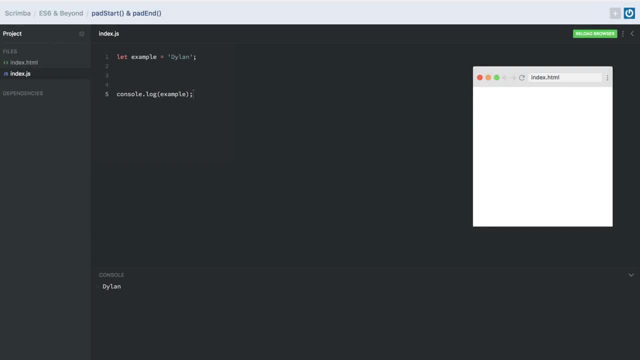 JavaScript gives some more love for strings with the pad start and pad end methods. What this does is it gives us a way to add values to the start of a string and add values to the end of a string, depending on how long the string is. 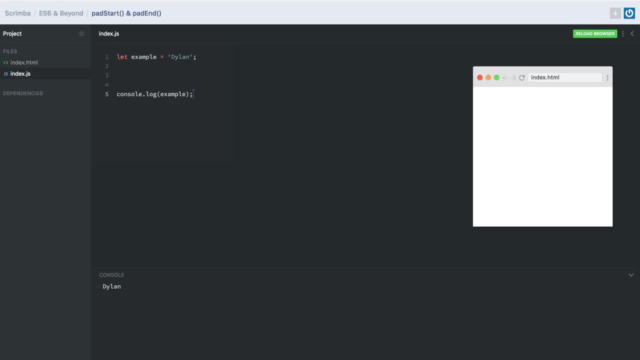 So let's take the example here, which is my name, which is five letters long. What we're going to take in, what we're going to call on this, is the pad start method, And this is going to allow us to put in an integer. 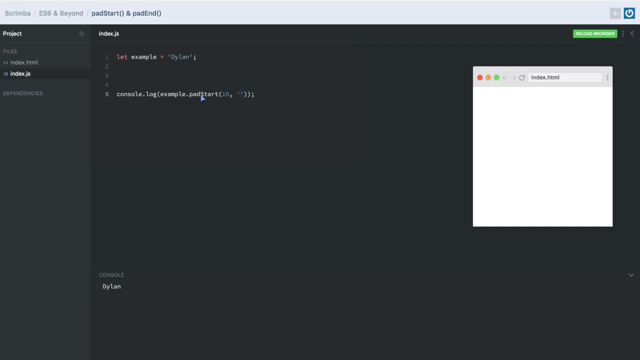 in this case 10.. And then we're going to follow up. Let's just start, Let's throw in the letter A And you'll see here, when we console log it out, we get five A's and Dylan. However, let's say we space this out like so: 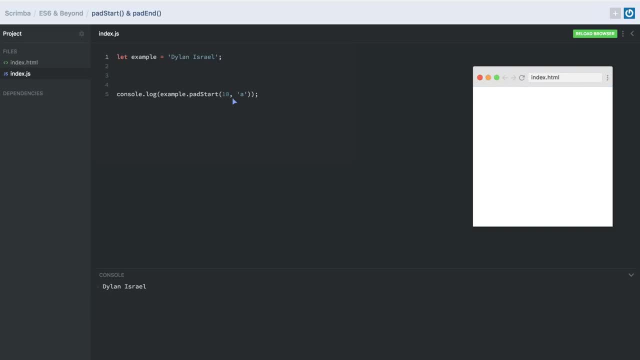 and we put Dylan Israel. We're just going to get Dylan Israel. There's no room left to add values onto our string And vice versa. if we wanted to do it with end start, it's going to work in a similar fashion. 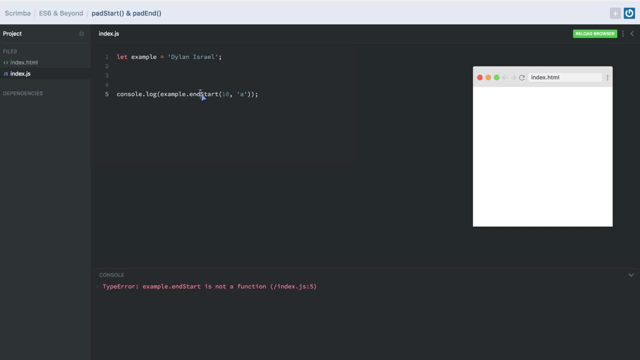 So we're just going to add it onto the end And, excuse me, pad end. I don't know why I said pad start, Pad end, You'll see. okay, there's no values here And if we remove Israel, 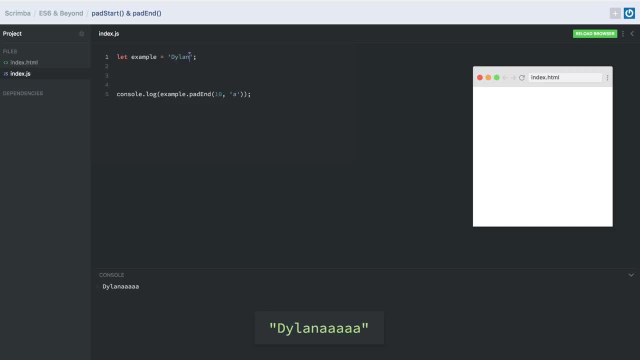 we'll have five values left. Then we'll add Dylan A to the end of the string, A little bit of fun. I haven't found a use case where I would use pad start or pad end, but it's definitely worth mentioning. Probably help you on some of those algorithm sites. 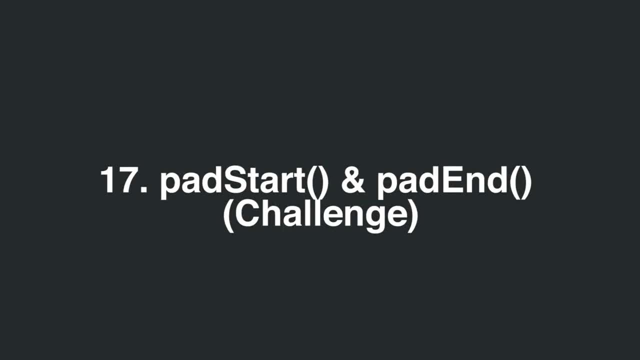 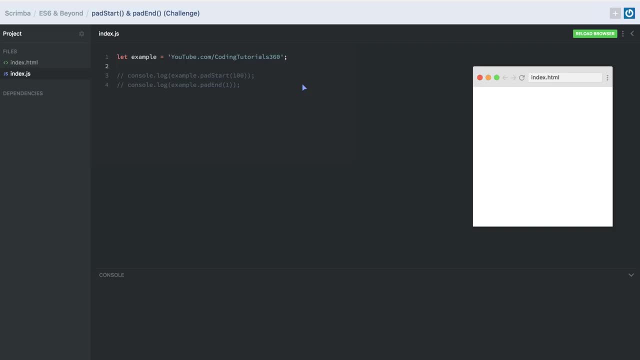 where you're practicing a little bit as well. So one thing you may not have noticed is that, or known, because I didn't mention it yet- is that you can actually pass in just a number here, The second parameter that we've been passing in. 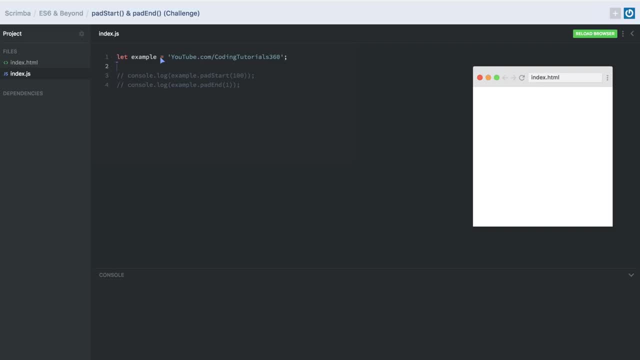 with the string is optional. So let's take a look at my shameless plug right here. YouTubecom slash ContourOS 360 string, which is a very long string and a very great YouTube channel, But besides that, you'll see that we have a pad start to 100. 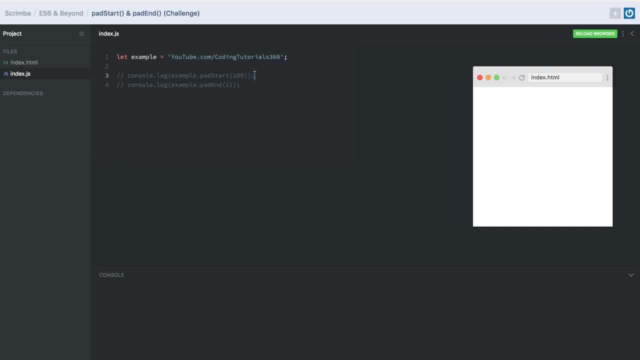 and a pad. end to one. What do you think is going to happen to our string when we do that? Did you come up with some guesses? If so, and you guessed that it'd add an empty string, you would have been right for our 100 one, right here. 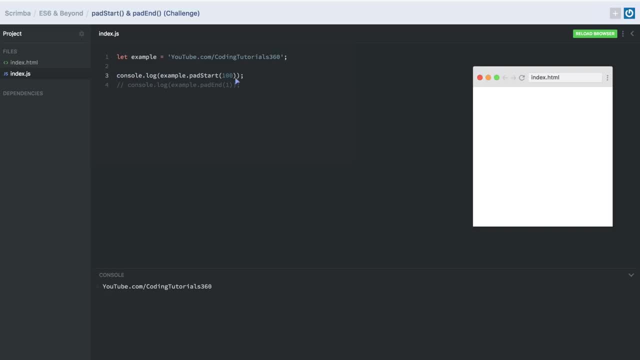 And you'll see. now it's going to print it out. We get that empty string but it's actually going to print out. if we call dot length on it, you'll see the length of it's 100.. There's like 80 empty characters on here. 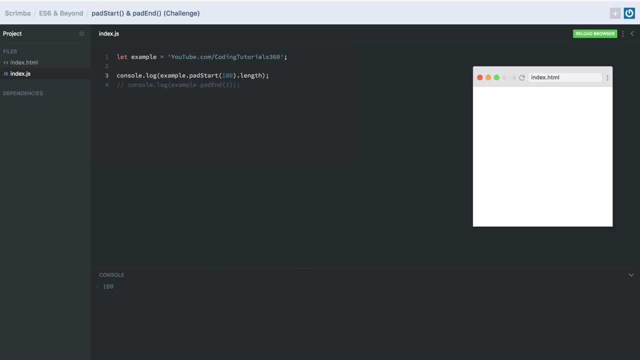 Just the editor here is too smart to know not to print all 80 of those. What about pad end? Well, in our case, it's just going to ignore it, right? Because our string is clearly longer than one empty character, and thus it prints out appropriately. 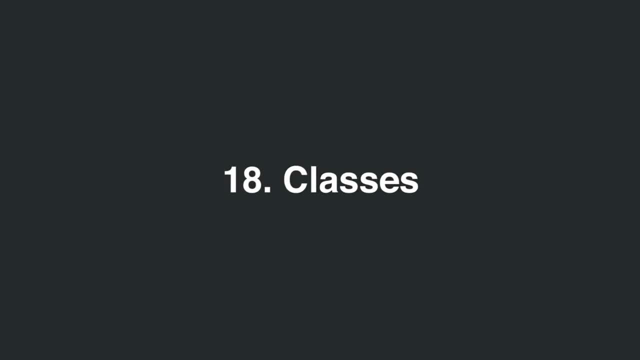 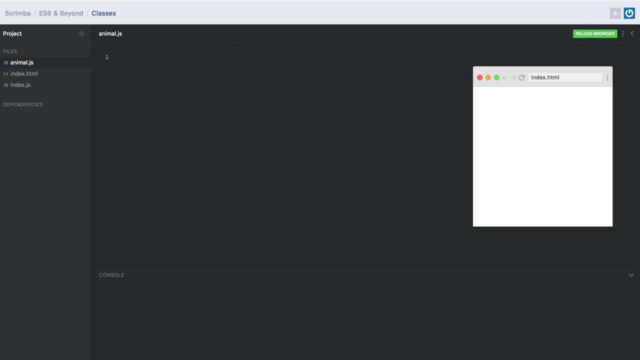 Classes are a great addition to take JavaScript to be in a more object-oriented way, And what we're going to do here is we're going to find a class and showcase some of the things that you can do with classes, how they work. It's going to be one of the longer sections. 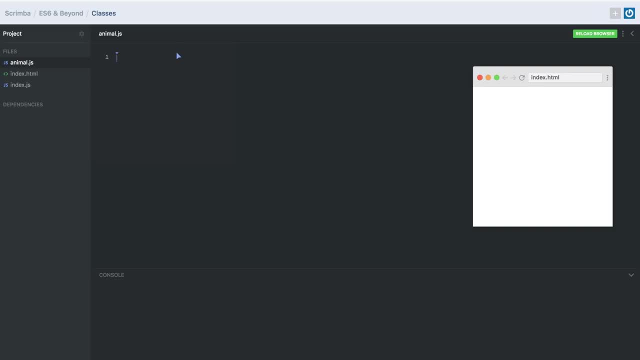 of this course, but stick with it. It's a really important concept. So let's start by jumping into our Animaljs file and define a class. You do that with this class keyword. In our example, we're going to use an animal. 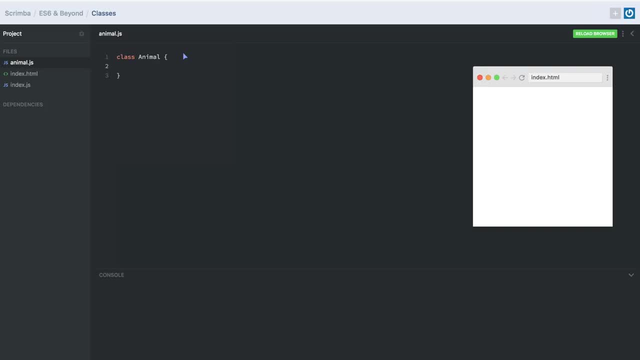 because I have three cats and I love animals. So we've defined a class here. It doesn't do anything yet, but we need to build an instance of this And to do that we have to set up something called a constructor, So our constructor here. 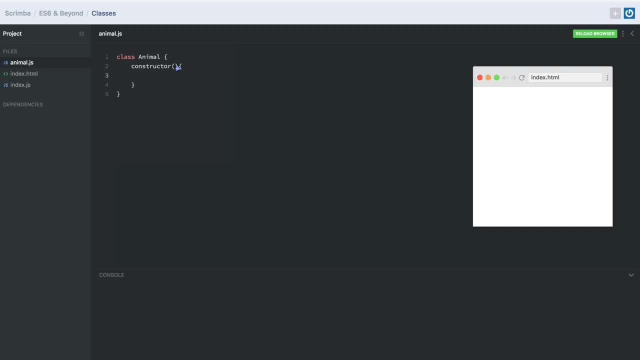 essentially sets some values when we create it. In our case, maybe an animal has a type and we'll also say it has- I don't know- legs. Every animal should have legs. And we'll go from there And we're going to use this keyword. 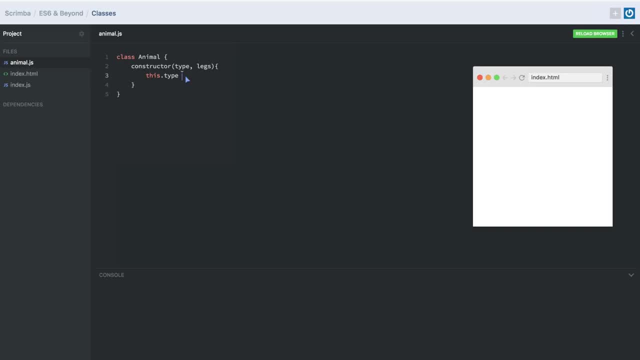 and say: look, thistype- meaning that this animal class has a type- is equal to the type that we're passing in, and vice versa, thislegs is equal to the value that we're passing in when we create our object. So the constructor here 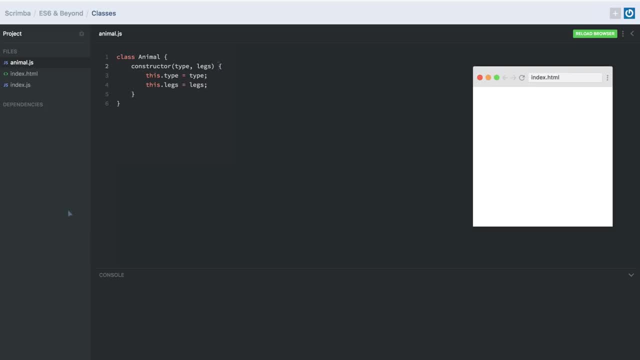 is really just assigning those values to our animal class. Now I think this will make more sense if we use it in an example. So let's go ahead and we take what we learned with the export- remember export class animal. So all we have to do 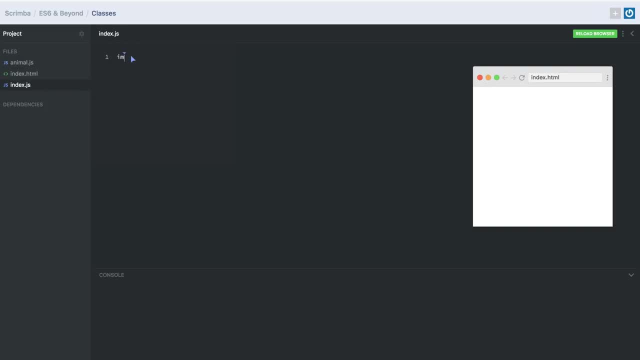 is, throw export on here. And now we'll jump into here. We'll go ahead and import animal from slash animaljs And to create an instance of a class, we go ahead and just create a variable here And we'll say: 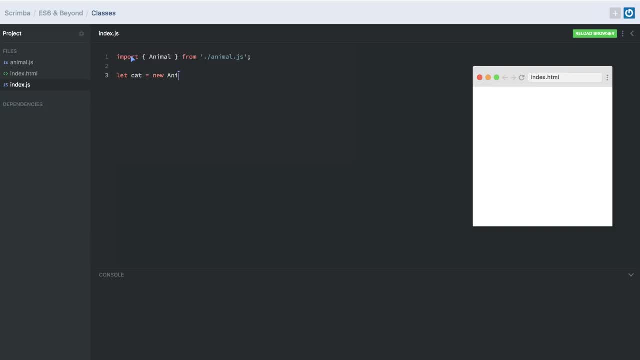 let cat equal new animal. Now when we go ahead and we're going to get an error, we go ahead and consolelog cat, you'll see that it's telling us. I'm surprised it even printed that. But essentially what the issue is here: 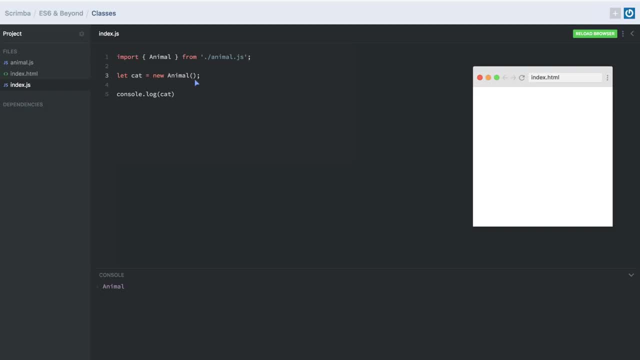 is that we need to now go and add some values. So maybe we have a type- we'll say cat and legs, we'll say four, And we have access to this animal. So if we say cattype, what are we going to get? 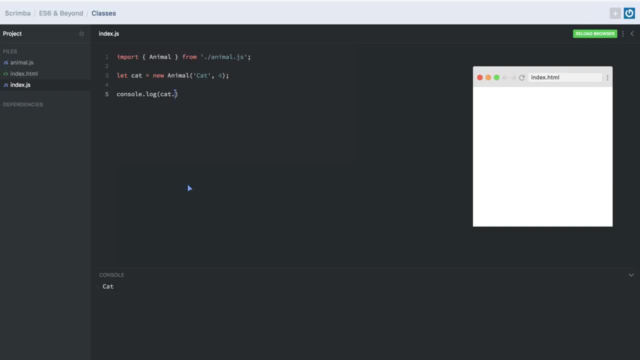 We're going to get cat right. If we say catlegs, we're going to get legs, And so we have access to those properties and they're being set via the constructor. here The constructor is setting these values that we're passing in. 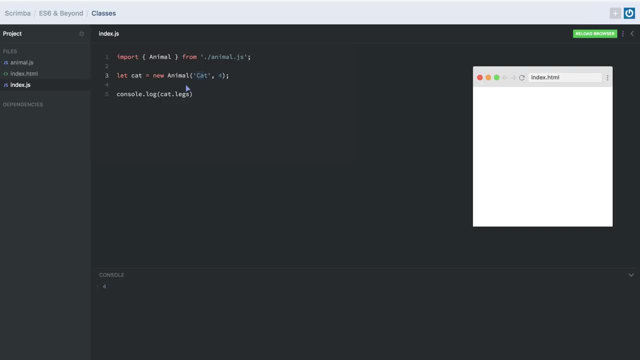 for our animal class. So we've already shown you that we can get values, but we can also change them, and change values relatively easily without having to change anything. All we have to do is say cat, And you'll notice how it's bringing it up right. 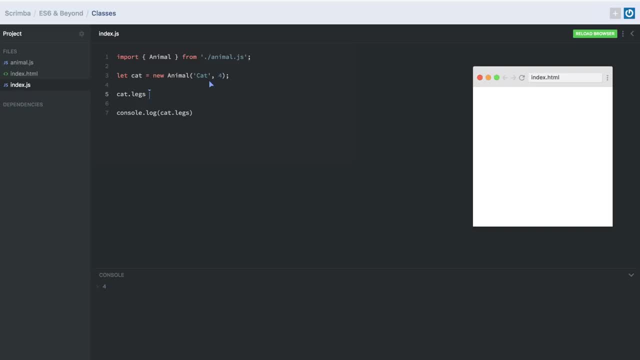 Legs, or type the legs And let's say: heaven forbid, our cat lost a leg. now they have three. We can then reset the value of that, just as we would with any other object. We can also define functions in our classes, And you'll see. 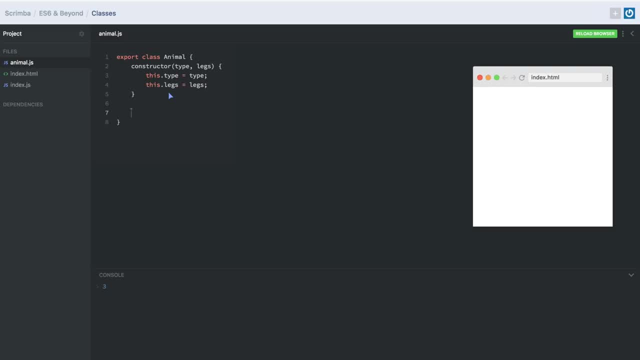 that we aren't going to use the function keyword for this. So let's say we define a meow or a make noise function because this is a generic animal class, It's not necessarily for a cat And we'll take in a property. 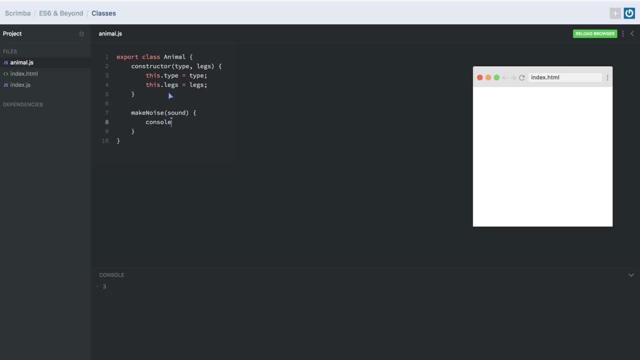 We'll just call it sound And then we'll go ahead and consolelog sound. And while we're at it, why don't we go and practice a little bit of the default params, because we covered that earlier, And we'll say meow. 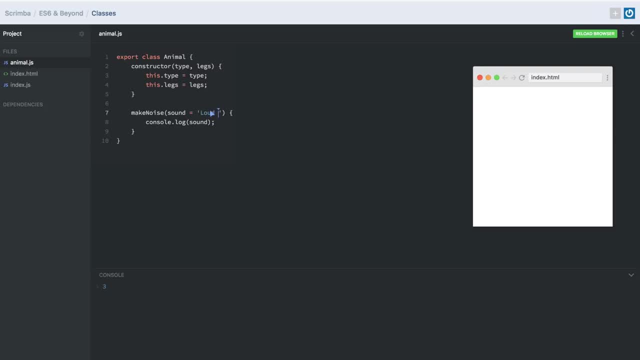 We'll just make the assumption. Actually, we'll just say: loud, Loud noise. There we go, And that should work just fine. So now we'll go to indexts And we can say: catmakeNoise, It's going to consolelog, loud noise out. 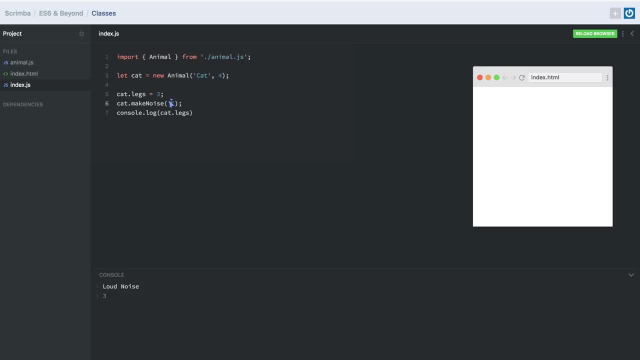 from the function that we passed in And of course we made it that optional parameter. So if we do pass meow in, we'll now get meow from our function that we've defined in our animal class. Static may be a new concept. 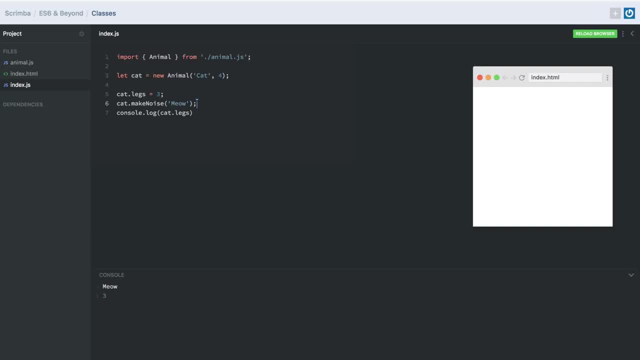 for those of you who are not familiar with classes and object-oriented programming, And what static allows us to do is essentially create a function in our class, in our animal class, in this instance, where we don't actually have to create an instance of animal to use it. 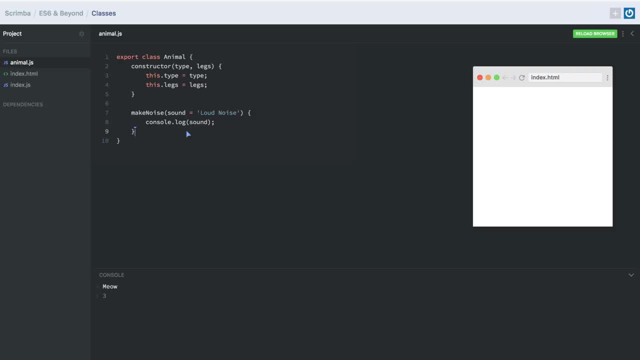 This is often what happens when you're creating a large library or you're importing someone's stuff and you don't have to create an instance of that class. So let's create an instance and create a static And let's say we just want to say return. 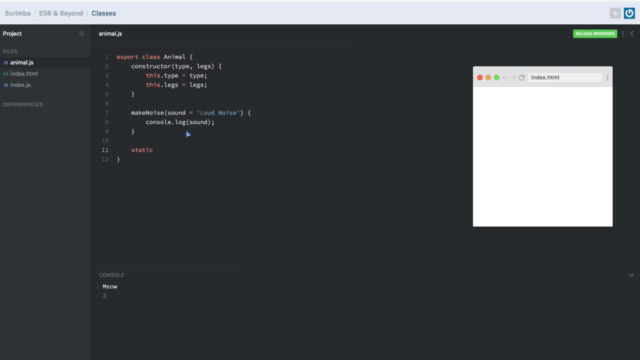 All we want to do is return 10.. It really can do whatever you want it to do And we'll say: return 10.. And that's a function. And in here, all we want to do is return 10.. Not the most impressive function. 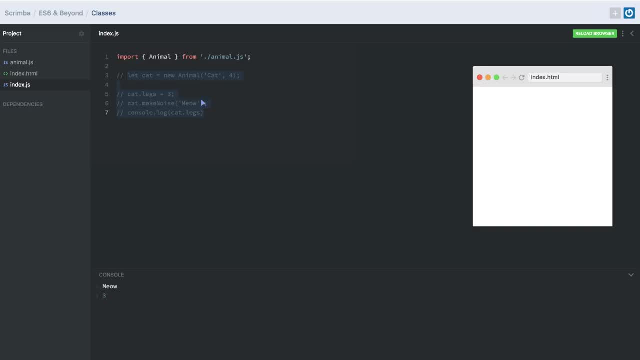 but if we were to comment all this out now and all we wanted to do was consolelog animal and then say return 10, you'll notice that it's going to work just fine. Excuse me, It's a function call. 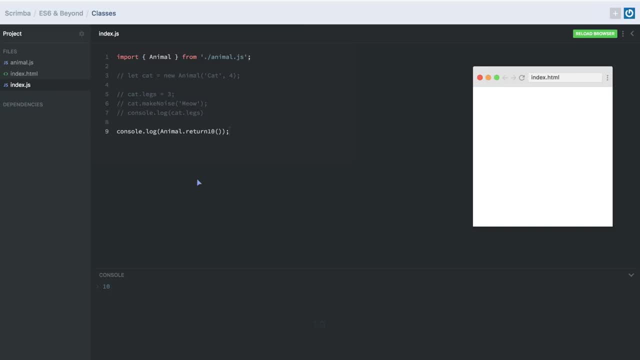 so we have to use that. You'll see, we actually get the number 10, and we never had to instantiate the class to use it. So these are really functions that you want to write, that you don't need an instance or anything too too unique about it. 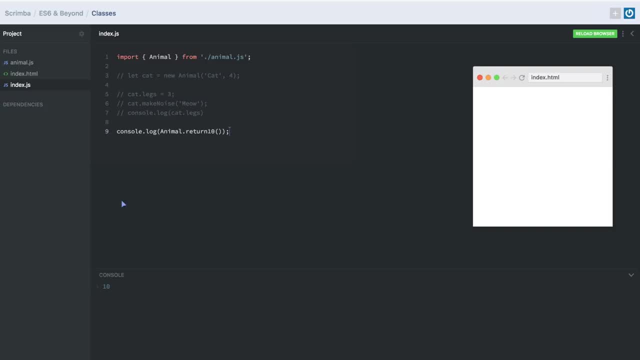 and that it's just going to take in some properties, perhaps, and return some data or run some. Another great option when it comes to classes is the ability to create a get method. So what is a get method? A get method is really a property. 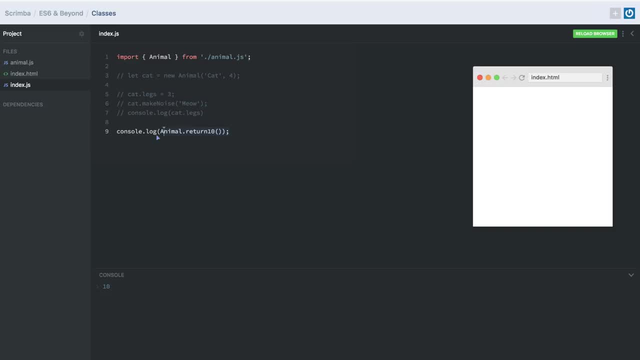 you want to create only to return some value. So let's go ahead and console out our static or get rid of our static method here and comment this back in, And we'll go ahead and just delete this. No need to do that. 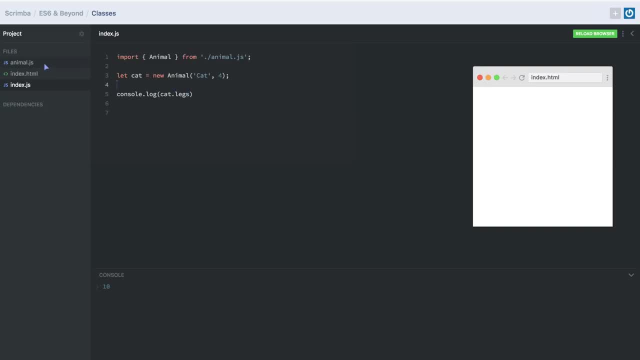 We all know that works at this point And we're going to jump into our animaljs file and we're going to create a get And you'll see, you'll notice the get keyword in front of our function call And in here. 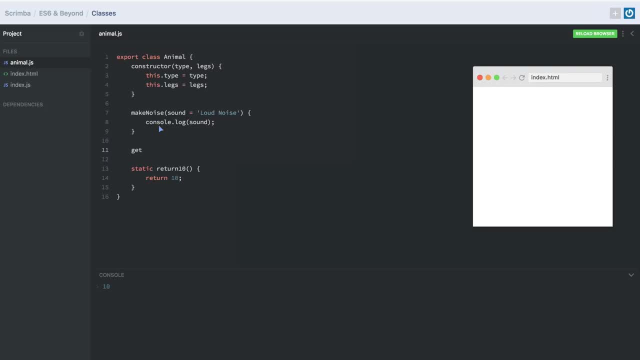 all we're going to basically do is return a string that says the type and the legs. So maybe we'll just call this metadata And we're going to return with the backticks, Say this dot type, And let's make this look a little nice. 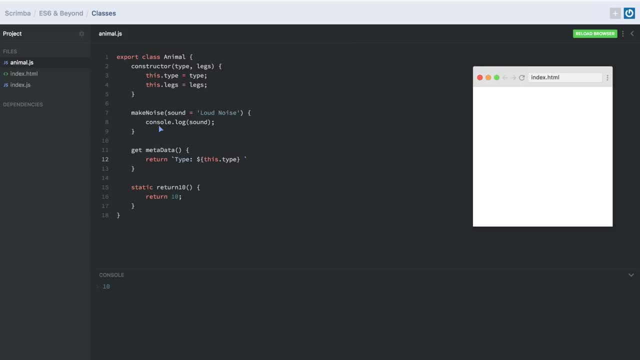 Type colon space And then we'll say: you know, maybe comma legs, This dot legs, And so this get, this getter here, will allow us to treat this as a property on our object. So when we jump back into indexjs, 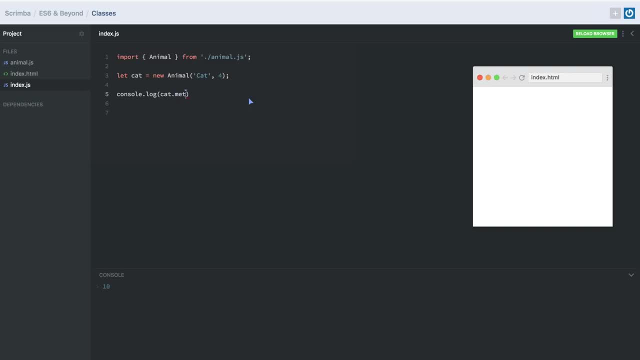 instead of printing out legs here. if we created a get, we can now get the metadata on it And you'll notice that it'll print out. So that's another thing that you can do. It also gives us the ability to maybe say: 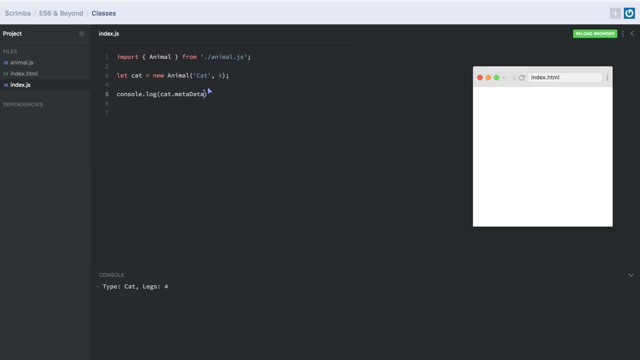 call functions in there hide a little bit of our class from the, from the user, if we want to, But this is another great option when it comes to working with classes. Now, as you continue to dive into classes and the object oriented programming approach, 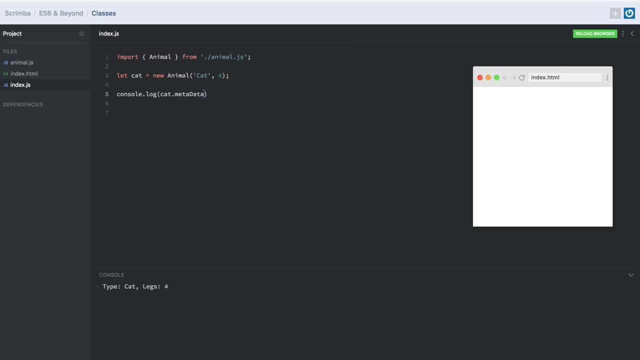 what will happen is you'll sometimes have classes that will share properties or be very similar, right? So in our instance here, we created this animal class to replicate a cat, but let's say we had a dog and we had a cat, and we had a mouse and all these sort of things. 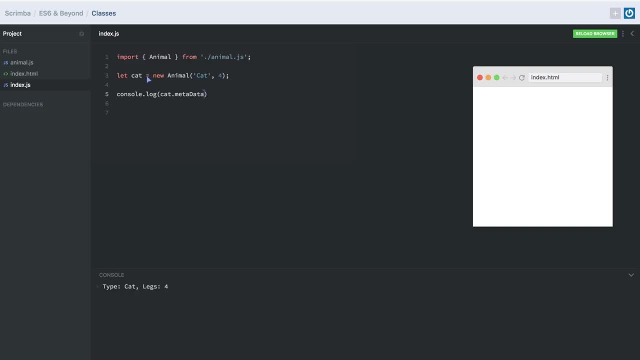 There, there may be a cat class, There may be a dog class, There may be a- you know- a mouse class, And. but we wanted to inherit some of this animal class and not have to rewrite all of our logic. Well, we could do that by defining a new class. 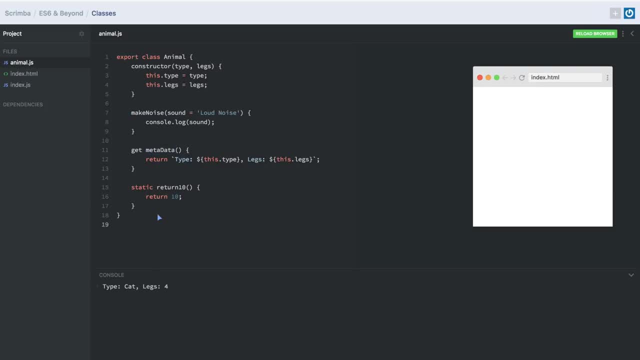 and we're going to do it in the same file here. but typically you'd probably have a different file, you'd probably have a different folder and then just import this animal class. So what we want to do is we want to export a class. 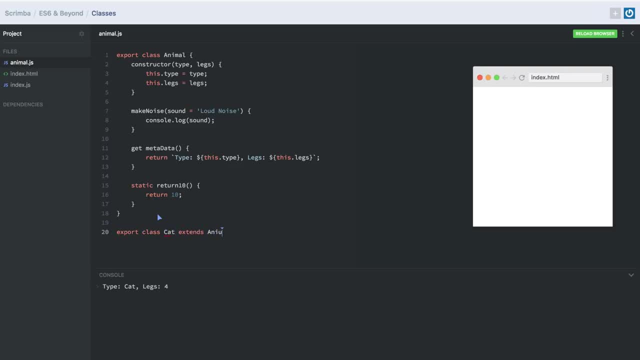 and this case is going to be cat, that extends the animal class That's going to allow us to inherit some properties from that, as well as overwrite the ones that we want right And the one that so we're going to inherit this constructor. 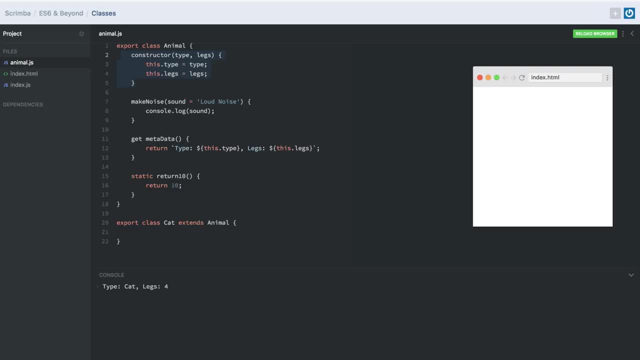 We're not going to have our own constructor, but if we did, we would. we could do that, but we'd have to put some keywords. I'm going to show you this, but we're not going to use it right now. 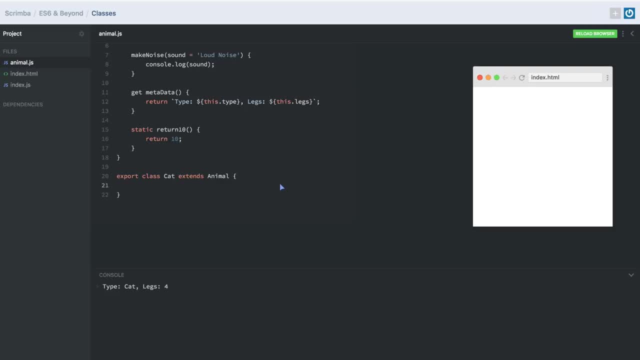 So let's say we wanted to have a constructor in our cat class here, like so, and we're going to have it also take in the same parameters, which was type and legs. But we also wanted to have a parameter tail here and we'll maybe just make it a Boolean. 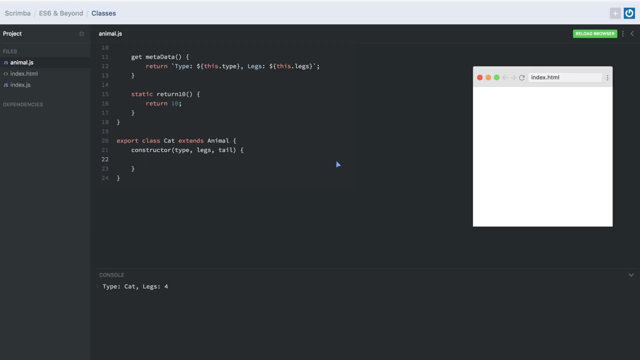 Perhaps a cat got its tail ran over and no longer has a tail. So it's a true or false. but when we use this constructor, when it's being extended out from a parent class- in this case animal, we're going to need to use the super keyword. 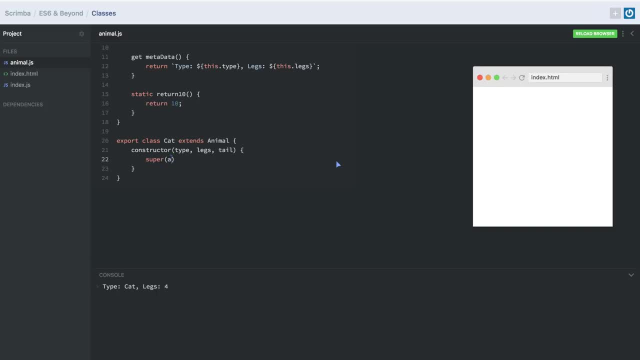 to let it know that, hey, pass in, pass in the values that we have here, which in this case is type and legs, And then we would also go about it the same way here, where we'd say: this dot tail is equal to tail. 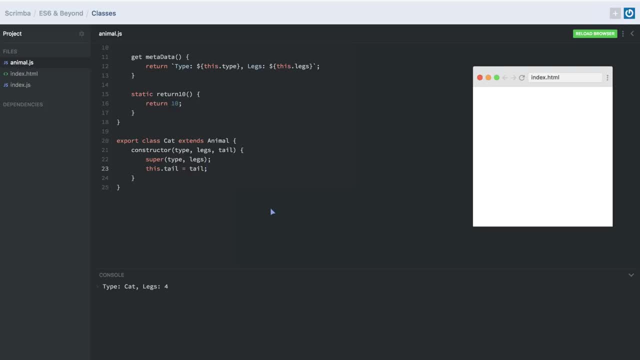 Now, we're not going to do that in this instance, but we want to bring that up, that you may run into some issues as well, as you can use super to call some functions from the parent class. But I just wanted to mention this. Let's go ahead and keep moving forward. 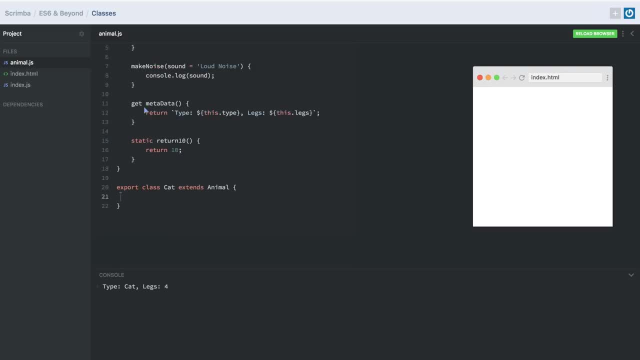 and see how we can override a method. In this case, we're going to override this make noise method And we're just going to make noise and we'll just still have it sound and we'll set default equal to meow, Because it's cat right. 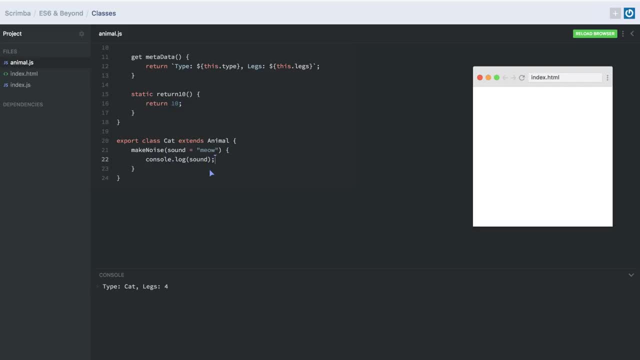 And all it's going to do is consolelog the sound, And so what's going to happen here is these are both named the same and they have the same amount of arguments, And because cat extends animal, we can overwrite this function in our cat class. 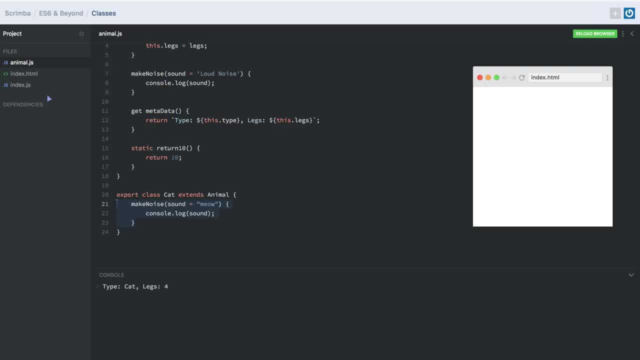 to make it more unique and more specific to what we're doing, while still have access to these other methods. So let's jump back into the indexjs and import our cat class And instead of cat animal- excuse me- we're going to import cat. 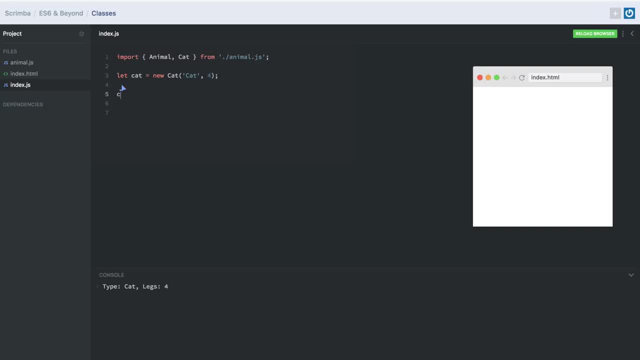 The first thing we're going to do here is we're just going to say: hey, catmakeNoise, And we'll see that it will do the meow and it's not going to do the loud sound as before, because we've overwritten that class. 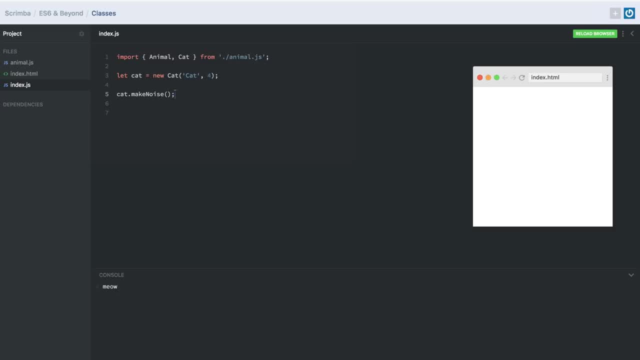 overwritten the parent class in our child class, cat. One last thing I want to notice. we didn't really showcase it, but we now, even though we're using our cat class, we've actually inherited the properties and the types and the methods from our parent animal class. 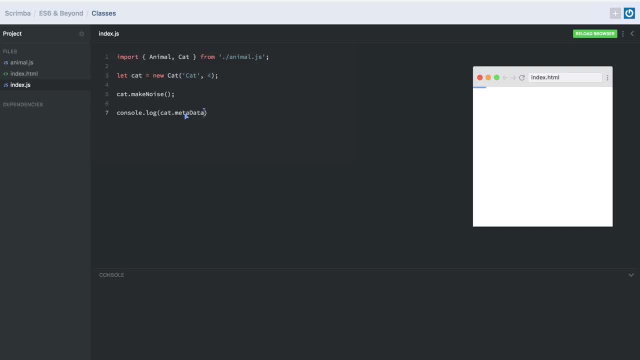 So we can get that metadata. for instance- And you'll see here we're going to get the type is: cat legs is four. So as you're starting using this object-oriented approach, I would suggest using it lightly. A lot of times people create very tightly coupled parent. 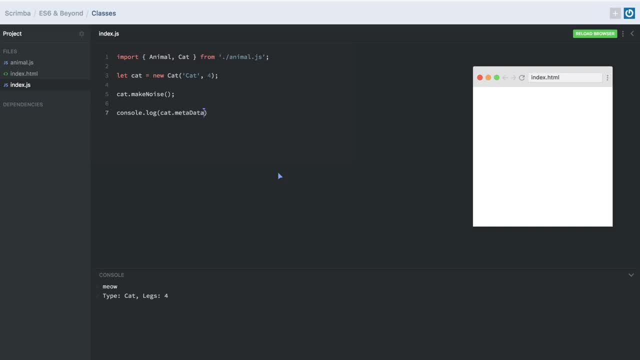 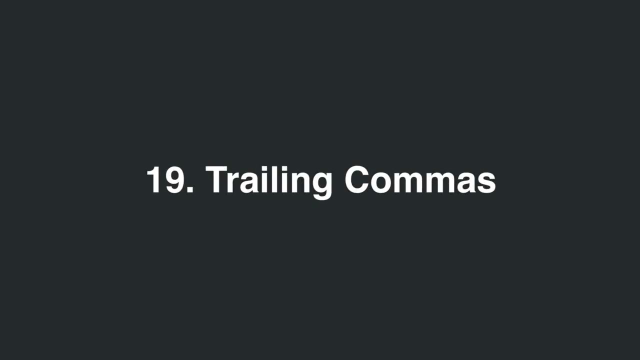 and child classes, and sometimes they should just be separate classes. But in certain instances it does make sense to extend your parent class out, And here is a good example of how we might do that. A debatable nice feature. I'm not too big a fan of this. 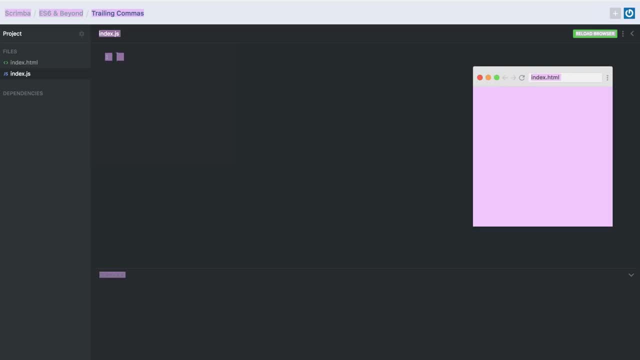 but a new feature added in ES6 is trailing commas. So in the past, if you had a comma that didn't follow anything, you would get an error. However, now, if we were to do something like define a function, we'll just call it add. 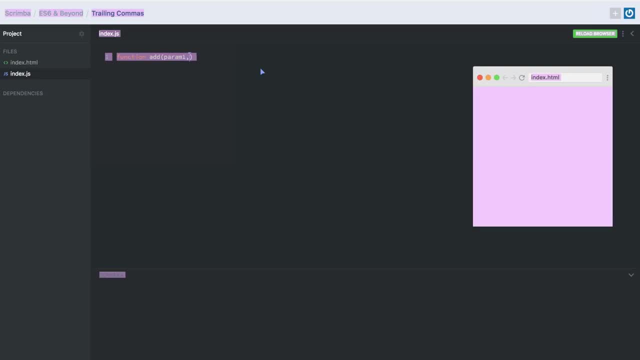 And we were to have, you know, param one, And then we had this comma. it would be fine. There wouldn't be any sort of logic error. That would work just fine. And same goes for objects, right? So let's say param one. we'll say: 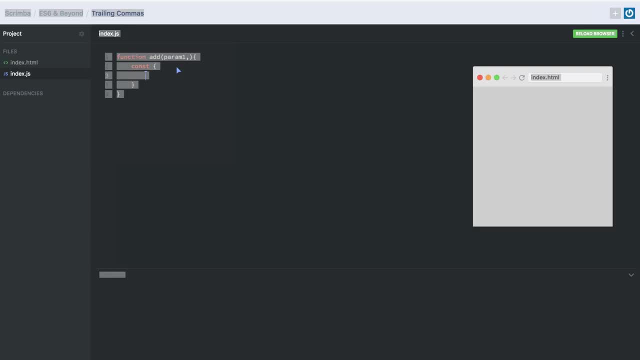 well, we'll just print out a const variable and we have name and we'll set it to Dylan. And then we went and set this trailing comma here. That would work As well. Oh, excuse me, This example equal to Dylan. 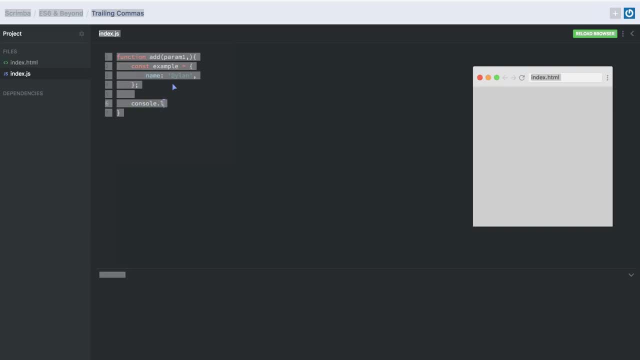 And then at the end here, all we did was just so that we could see it. consolelog, param one And just an example. consolelog example. But trailing commas are now something. we're not doing anything with this variable, we'll just call it though. 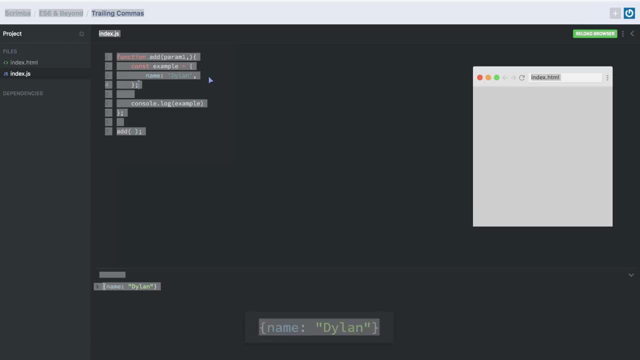 that we don't have issues with anymore, So you're allowed to have trailing commas. I'm not a super big fan of this. I think this is something that got put into JavaScript. maybe someone can convince me. but just to solve little tiny errors. 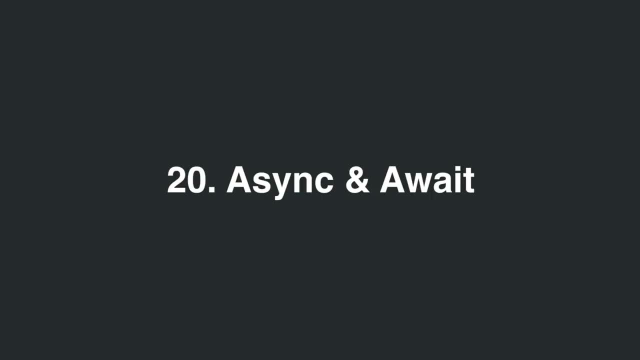 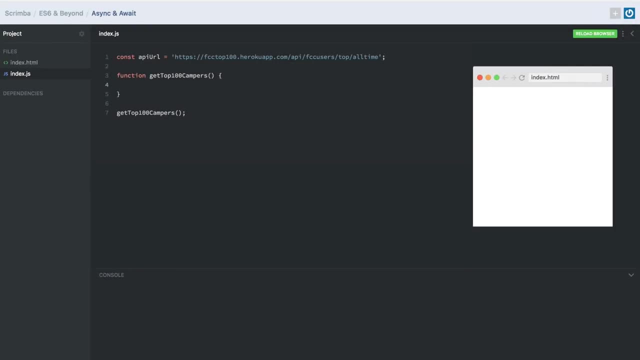 but it is something that's there. Be aware of it. So this is going to be a little bit of a longer section. We're going to be talking about promises, async and await and how they're all sort of related when working with them in the front end in JavaScript. 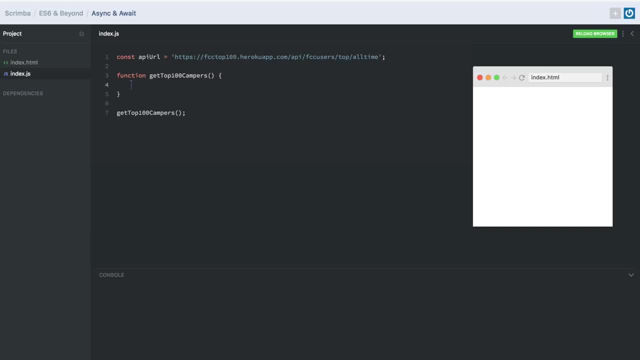 Let's start by talking about what we have on our page. here You'll see, I have this constant. that is a URL That's going to link us to a top 100 of the all time active users on freecodecampcom. 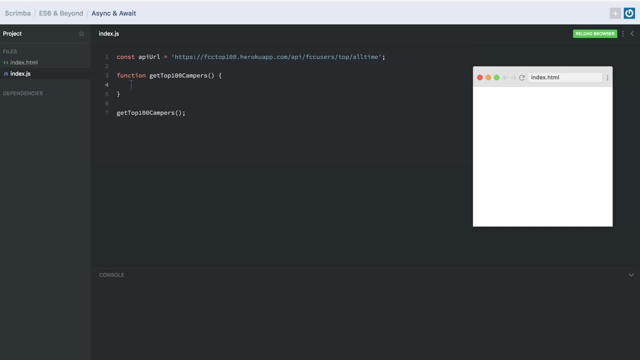 which is a open source JavaScript site. It's an excellent place, if you're. I believe they're actually going to be partnering up with Scrimba on some future stuff, So check them out if you're interested in that What we're going to do here. 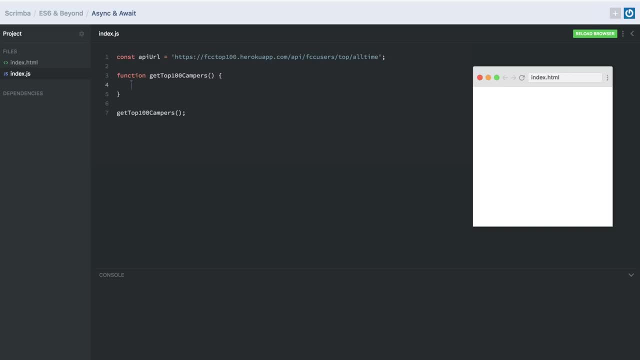 is, we're going to do an asynchronous call, We're going to go and do an Ajax call and we're going to be using fetch, which returns a promise, And we're going to showcase how to handle that, And then later on, we're going to showcase a little bit of async and await. 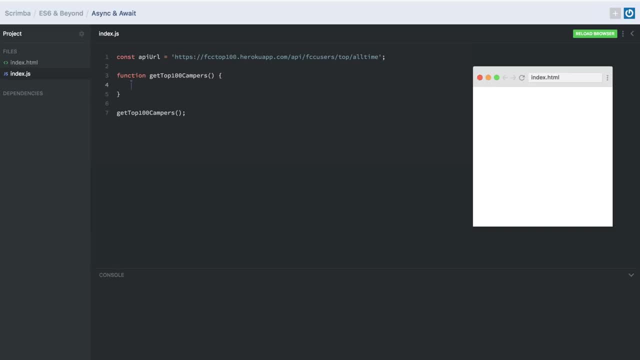 and how we might use that alongside promises. So let's get going here. You'll see we have our function. get top 100 campers. This is not like Call of Duty campers. These are the campers of free code camp. 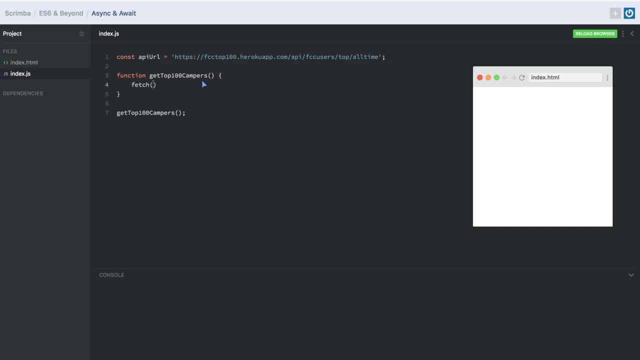 We're going to use the fetch method here, which what this is going to do. it's going to take an URL. This is really going to go and get the data that we're looking for, But there's a little bit more we have to do for that. 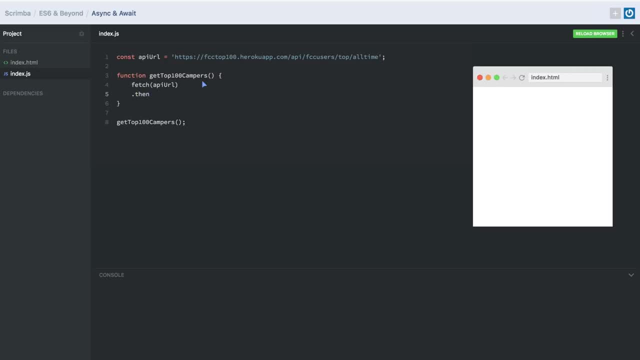 We have to call this fetch Then on it And you'll see here, when we say then is it's returning a promise of type response. That's what that means. And so fetch is returning a promise, Then we're going to handle that response. object. 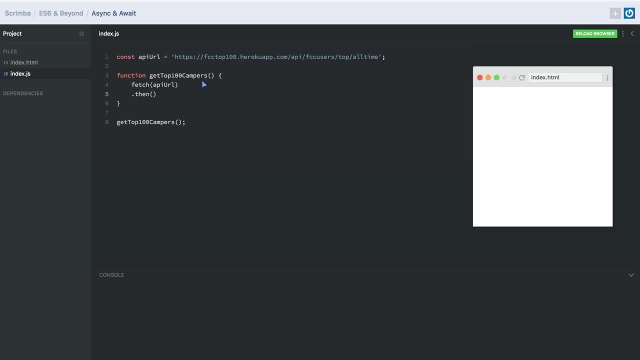 which we then said, hey, when the promise actually gets delivered, you can kind of think of like, hey, we promised to send you some data with fetch and then says, okay, when you actually send me the data, I'll do something with it. 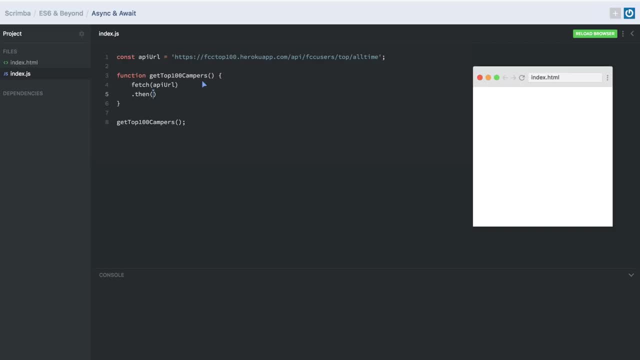 In the meantime, just keep running your code- That's sort of how asynchronous items work and how promises work in this case- And then says: hey, I'm going to give you a response. Just say R for response, And what we're going to need to do is first: 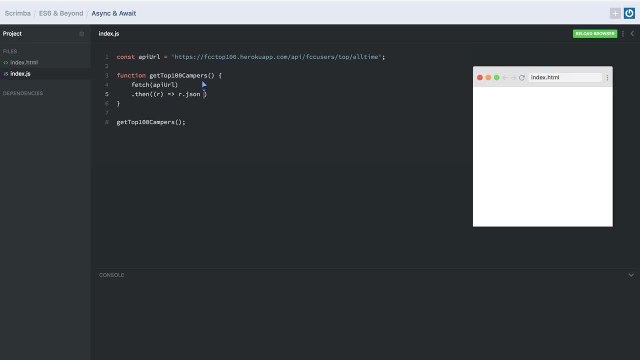 we're going to need to turn that into JSON, Otherwise we're not going to know what to do with it. Our computer isn't going, our JavaScript doesn't know what to do with it, And so we have to convert that promise into something that we can use. 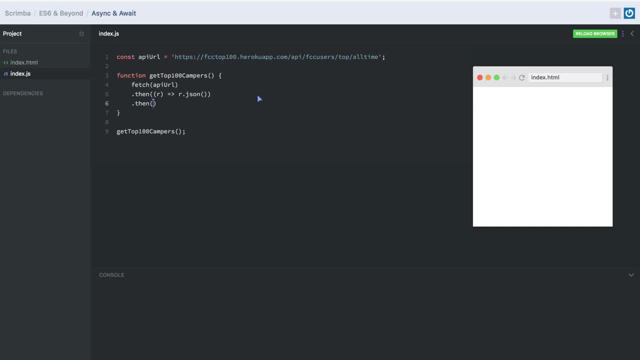 Once we do that, we can then take that promise, which is another promise, And we can- which, at this point, we didn't say it's JSON, And we can do something with that data. What do we want to do with it? 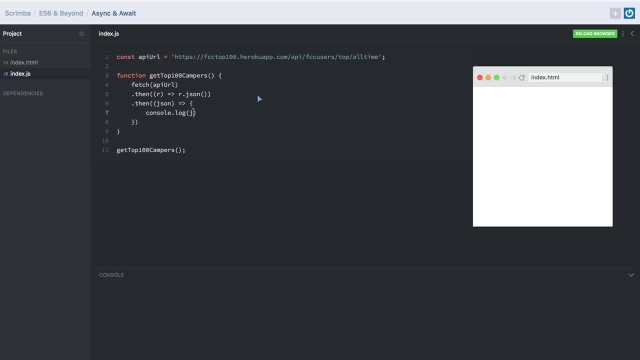 Well, let's just say we want to consolelog the first value of that JSON. This is going to return an array of a lot of values and put a little semi-colon here And we'll just see that our asynchronous call got set up. 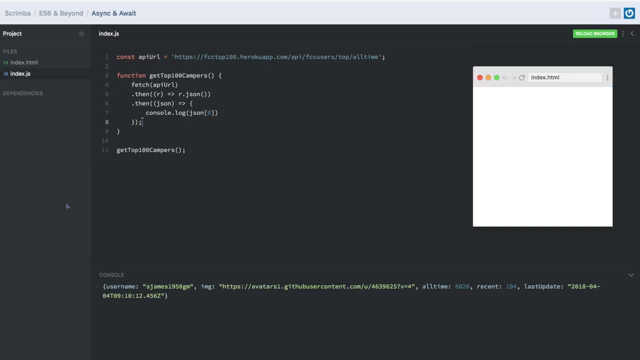 You can see here, we get this object from our Ajax call. Now, while we're at it, let's go ahead and showcase how we might catch this Ajax call in case an error is thrown, And that's I might've already given it away. 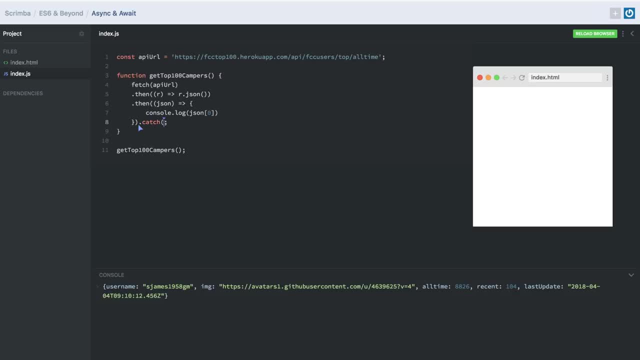 is by catching it. And so you'll see here: catch takes in a error result. In our case, we're not going to use it because it's going to look identical to the errors we would get in our application. So if for any reason, 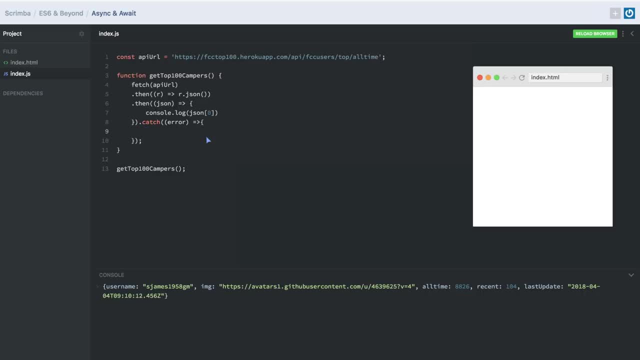 our server side fails on the fetch or converting it to JSON, we're going to get that error. So let's say that we wanted to. just consolelog failed, so that we know that it's firing off and we're going to go ahead and change this. 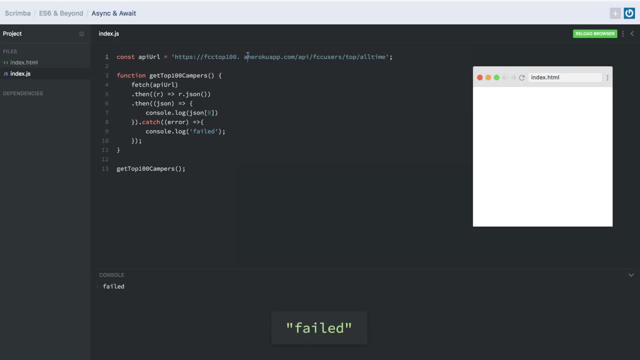 put like an empty space here and an A and save it. You'll see, here we're going to get this failed message and none of this is actually going to run because it failed immediately at the fetch standpoint. Let's go back and fix that. 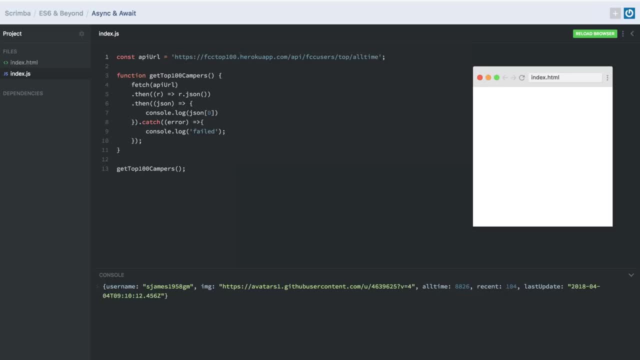 And you'll notice. now it's going to go ahead and print out our code. Let's move on. So, now that we've done our AJAX call, our asynchronous call, and we've resolved the promises and everything's working, let's show how we might do this with less code. 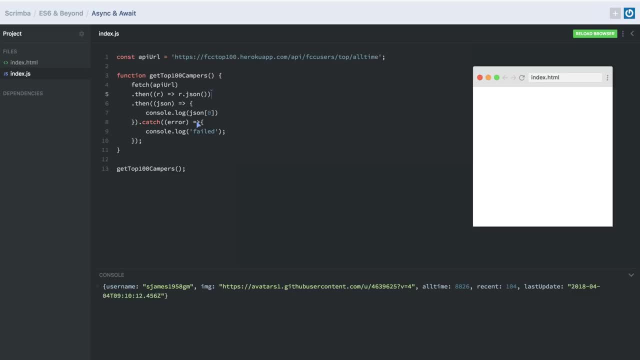 using asynchronous and await for an AJAX call. Now just keep in mind you don't have to use async and await or promises just for something when it's hitting a server. That's the most common instance. But let's say you had a timer. 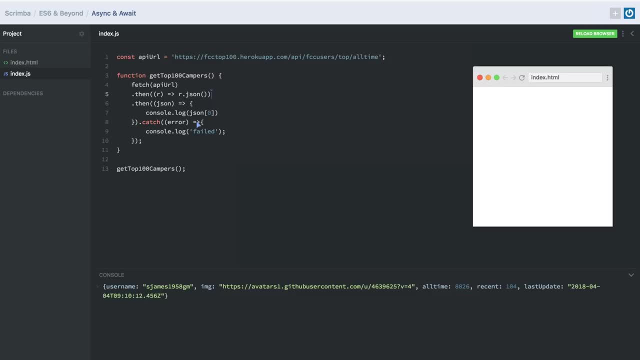 and it was timing out for three, four seconds and you wanted to have something to delay it. You might use promises or async await for that. I just wanted to show you the most common one, which is server calls, and get calls specifically. So let's go and fetch that data. 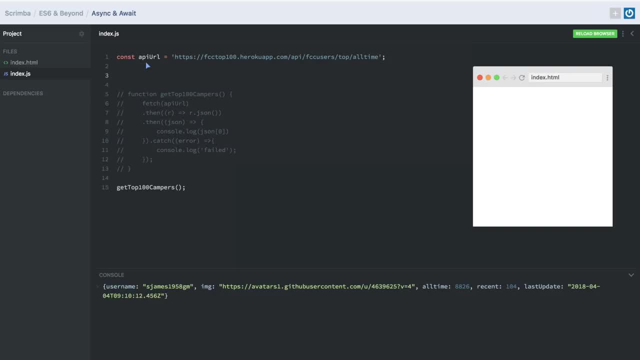 except, instead of doing it with the promises, we're going to do it with the async and await. We're going to define a function, same name as before and get top 100 campers. Now the way that you tell it that it's an asynchronous function. 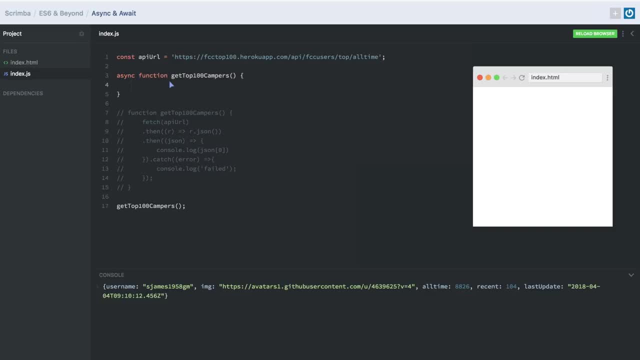 so what I'm going to do is throw this async in front of it Now. the JavaScript knows like, hey, there may be some asynchronous items going on in our function, and it will give us access to the await keyword. How we're going to get that data. 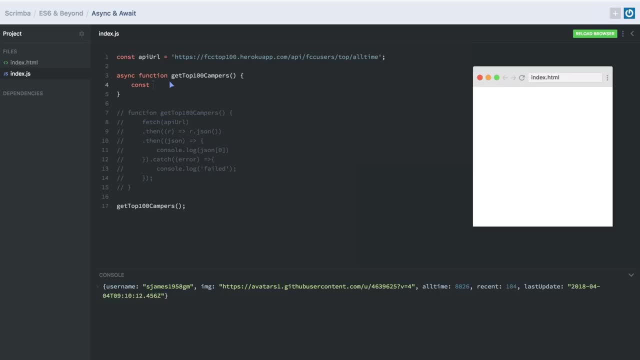 we're going to just define a const here and we don't have to store it. but I think it's a little bit easier. It explains the logic a little bit more And we're going to say: this is going to be equal to: 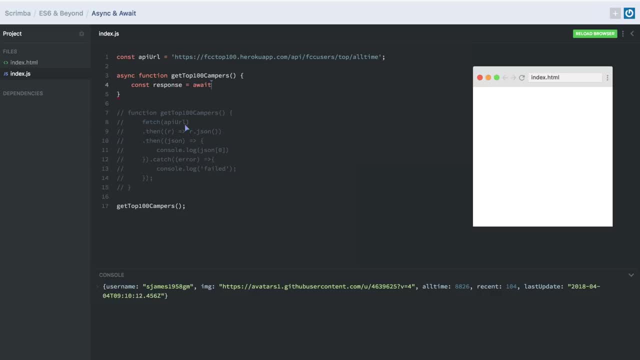 and we're going to do our first asynchronous call here, which is follow the logic, and follow the logic is fetching the data, So we're going to fetch on that API URL. Now that we've done that, and what that await is saying is: 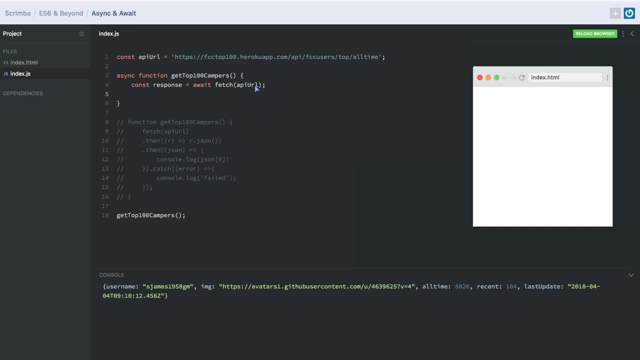 please wait until this fetch completes. Whether it's successful, whether it's not, please just wait until it completes. The next thing that we want to do: we go ahead and define a const here and call this JSON. This would be our second JSON. 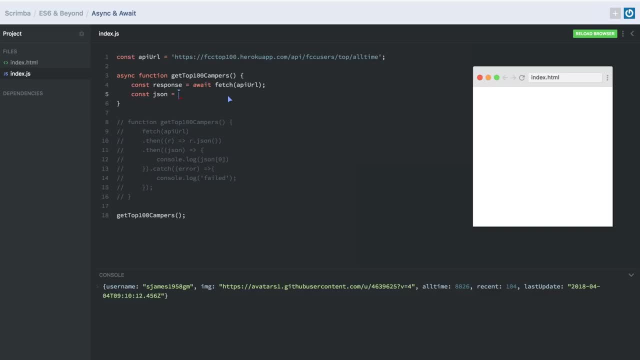 which is another asynchronous call, And we're going to set this equal to await, where we're saying please await our response, being turned into JSON, a response dot JSON. excuse me, Now that we have that, we have access to it, And it's saying: this line will run. 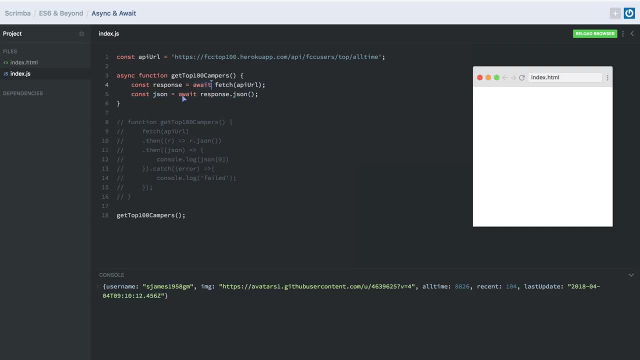 and it's not going to. this line will not run until this resolves. That's what this async and await is doing. And finally, at the end, here we can console, dot, log our JSON And again, we're just going to hit that zero spot. 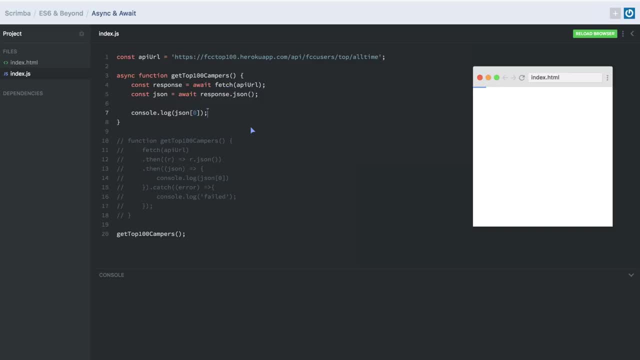 because the data is very large. So when we save, we'll get this nice asynchronous call. Now, if this wasn't asynchronous and we didn't have, or it wasn't an async and await, what would happen? here is our console log. 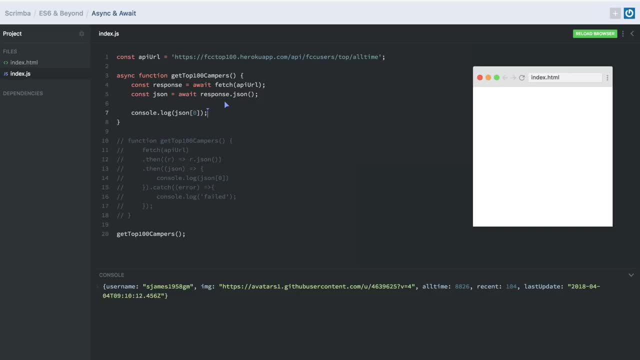 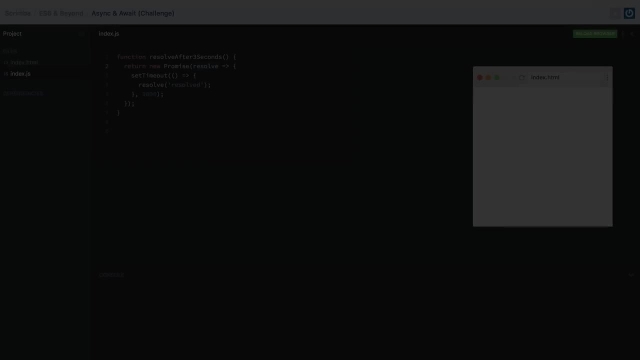 wouldn't know what JSON zero index is, because all the code would run synchronously just one after another and would not be resolved before we'd actually get this data. So this challenge is going to be a little bit instructional as well as really probably just by far. 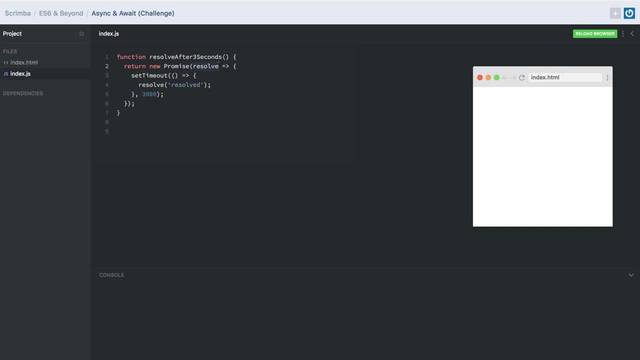 the most challenging one of the course. So you'll see here that we have a function called resolve after three seconds, And we showcase how to use promises in or having a promise being returned, but we didn't actually showcase how to create one. 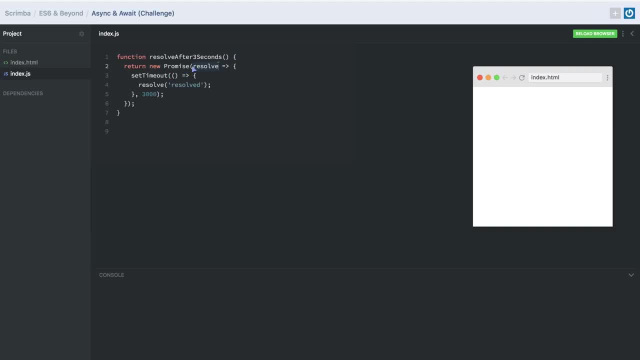 You'll see here that we are returning in this function a new promise, with the resolve eventually being the data that we're going to pass that back. In our instance, here we're going to set a timeout for three seconds, So promises are typically used with asynchronous calls. 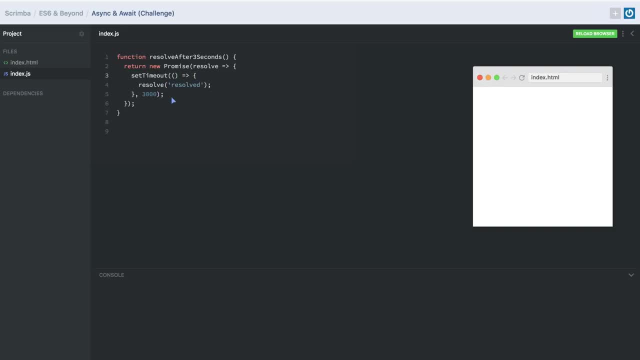 or things that take time, And in our case, that's what we're returning. So how might we solve this? resolving that promise to get that resolved set, And how might we solve this using async and await? Really, take a second to see if you can solve this. 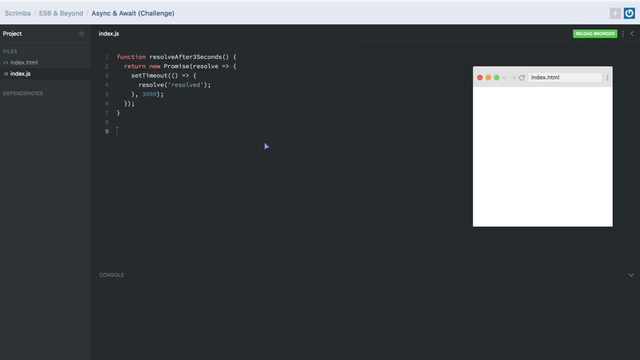 This is an important question. This is a fairly new concept. All right, hopefully you're able to solve that. If not, don't sweat it. This is a fairly new concept for most people. JavaScript has been synchronous for some time and now we're learning to work with it asynchronously. 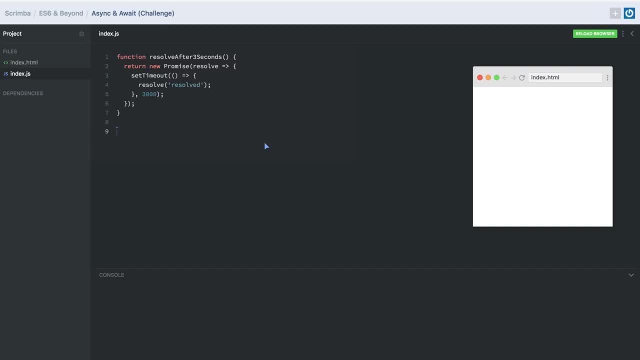 So how might we solve this using the promise then mechanism? Pretty straightforward, If you remember our last example: we are going to call our function resolve after three seconds, And then we're going to call the promise methodthen, which takes in our return data. 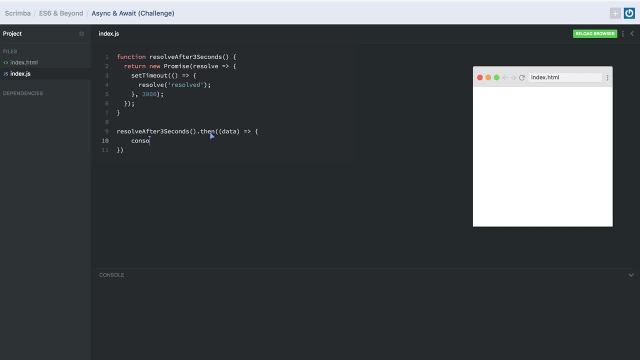 It's successful. And then we want to, in our case, just consolelog that data which will fire off after three seconds. right, 3,000 milliseconds is one second. So any day now, There we go, resolved The other way that we can go ahead and solve this. 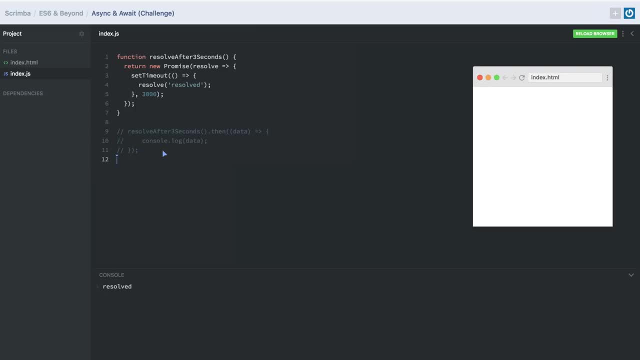 is, we can define an asynchronous function that uses async and await. So let's go and define a function. Remember, when we're defining async functions, we use the async keyword and we'll say: get async data. And then at the end, of course, 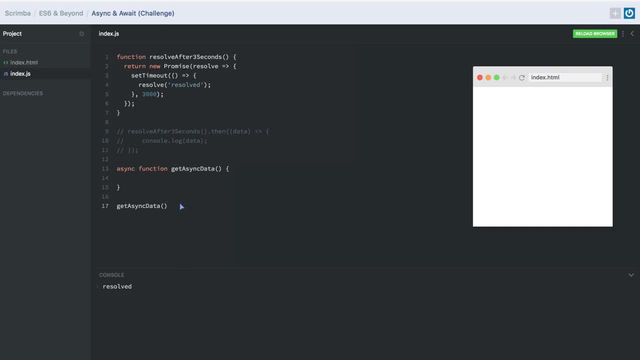 we're going to want to call this, to call this function, to go get that data. Now in here, all we have to do is await: await our output, await our data using the await keyword So we can store this in a result. 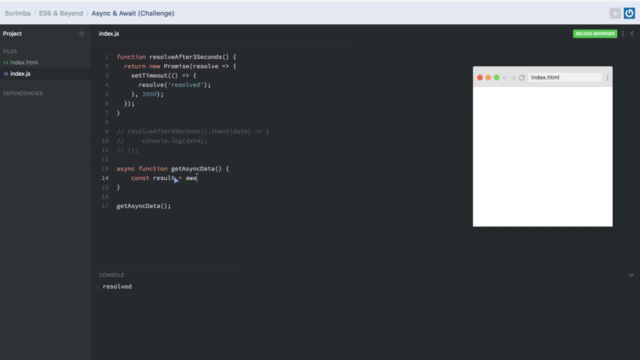 That'd probably be the most proper way of doing it: Consoleresult and then await the resolve after three seconds, And then consolelog that result, which will happen in exactly three seconds, And so our data here it's all going to flow properly. 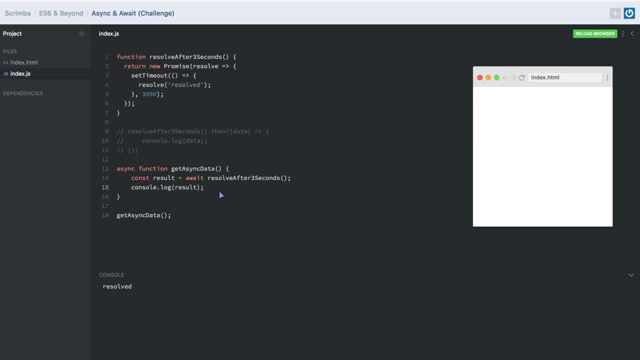 It's all going to work properly, And now we're handling getting data from asynchronous places, or from asynchronous endpoints, or, in our case, using promises with timeouts, And it's another way that we can use this and an important concept moving forward when you're trying to deal with databases. 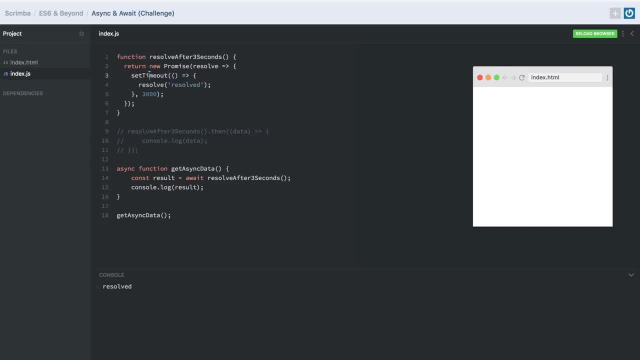 and getting data, receiving data. So I hope you found this helpful. So this has been a great addition to JavaScript. What they allow us to do is create a unique list. Now how might we go about creating a set? We can start by just creating a variable. 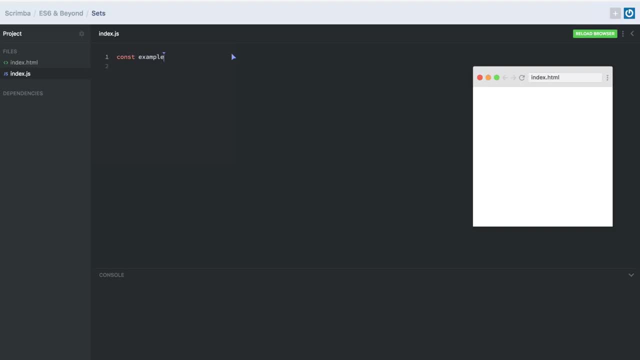 And go ahead and say const. We'll just say: example set is equal to a new set, And then inside here we're going to throw in an array And let's throw in some duplicate values. The reason for this is to showcase the idea. 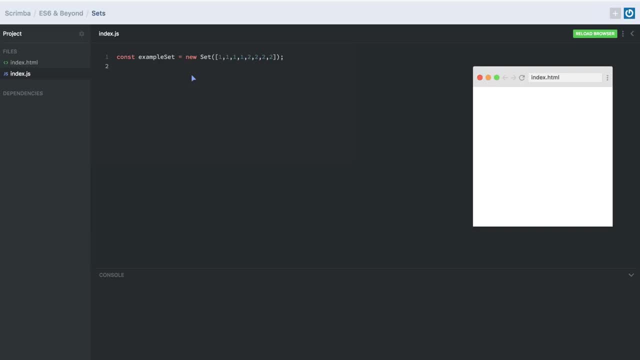 Also the way that Babel is set up in Scrimba right now. it doesn't fully work in terms of the way that it compiles to the console log. So instead of actually printing out the example set to C, it's just going to say set. 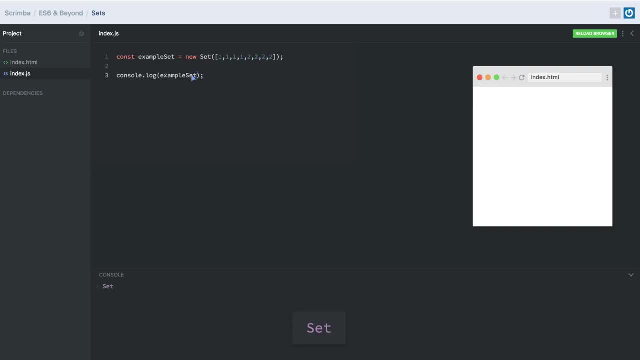 No way around that right now, at this time. But the idea you'll see right here, we have two unique values in here And that's all the set cares about The other values. they don't even exist. So when we want to see the size of it, 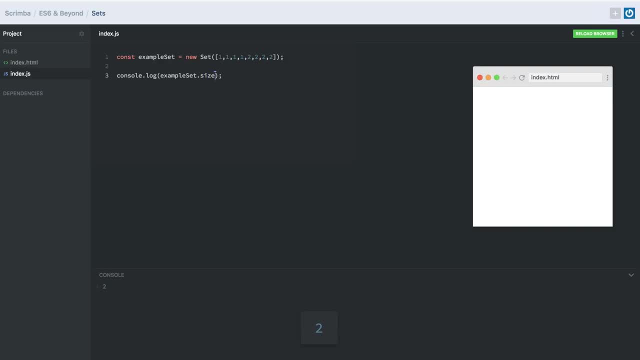 we can do it with the dot size. You can see there's only two. Now let's say that we wanted to add to our set that we have created here. We can do that with the add method And we could throw in a new value. 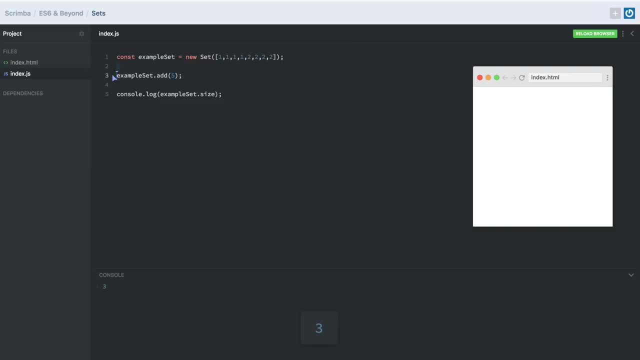 Here five, And this is going to add three And add works the same way, where, if the set already has a value, it's not going to add it, It's just going to basically ignore it. And we can chain these as well if we wanted to. 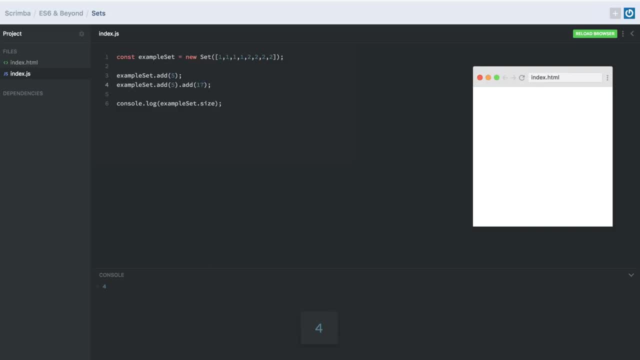 Let me go ahead and throw 17 in there And you'll see our set size continues to increase. You can also remove values from set using delete. One thing to keep in mind is a cool function of sets, in my opinion, anyhow- is that when you delete it. 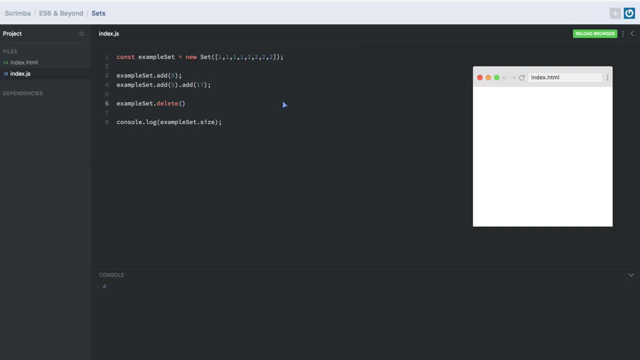 it actually returns a boolean of true or false, whether it was successful. So let's say we delete five And we're going to consolelog this out. What we're going to get is true because the five exists in there And you'll see right here. 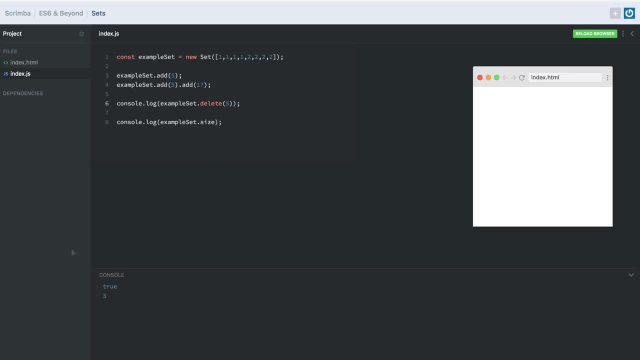 So then it of course removes it from our element. So that's another side effect of the delete method. We can also check if a value even exists in our set using the has. So we're going to go ahead and do that. 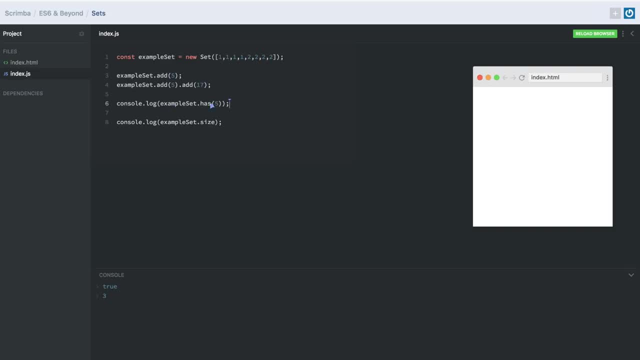 And we're going to say, hey, does this set have five? And you'll see, it does It's true, right, And our size is four. And then, last but not least, one more thing to mention is that we can actually clear out. 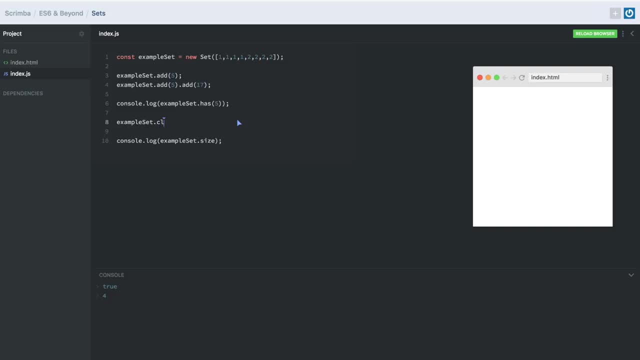 our entire set and reset it with clear, And then you'll see, our count here is going to be zero. The last thing I want to mention is that a set is iterable, So you can use things like foreach on it and four of, and all the great ways to do that.